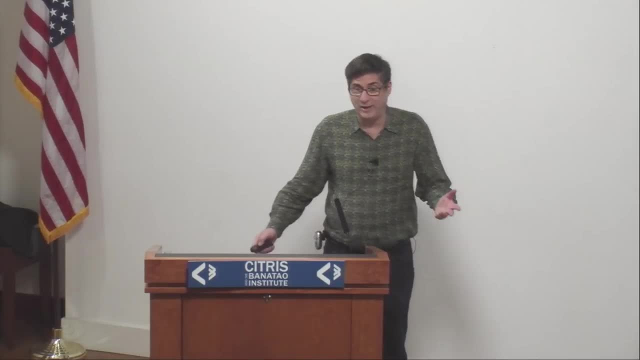 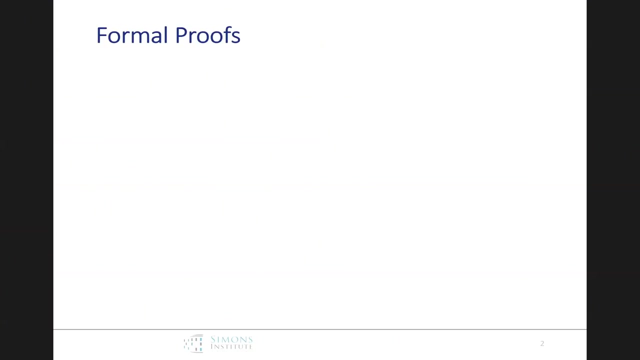 Thanks, Shafi, and thank you for coming, given the weather outside. So some of you the part of this talk will be quite old hat, but I hope there'll be interesting things for everybody in the talk. So I'm going to talk about the limits to proof and when we start, we start with formal proofs and there really are two people at the late 19th century, early 20th century. 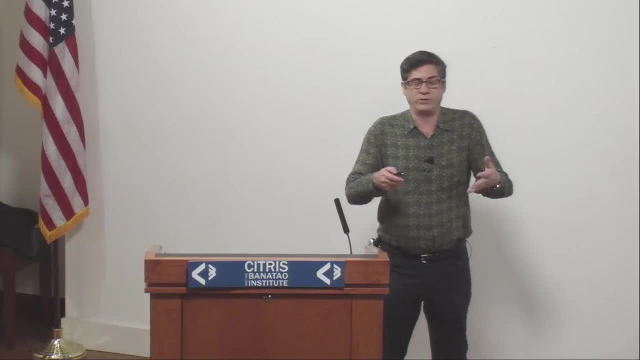 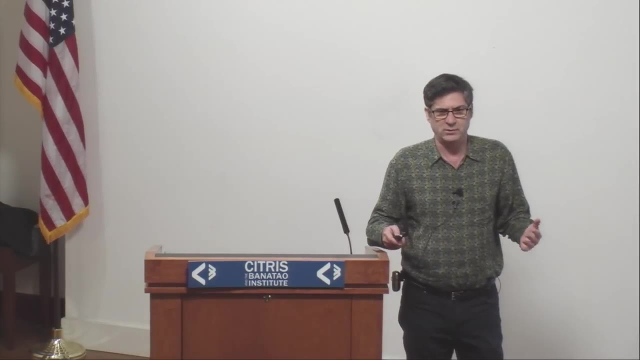 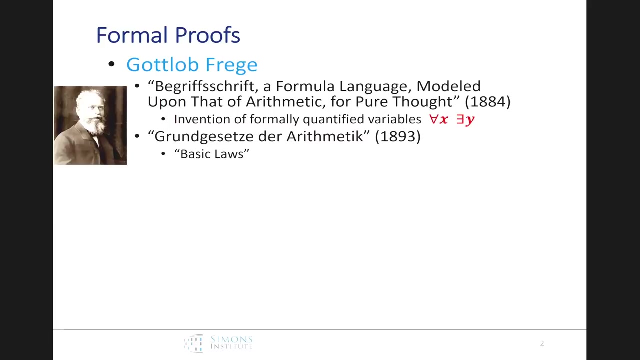 who really almost synonymous with the introduction of formal proof. One was a superstar in mathematics and the other is largely unknown or very little known. The little known one is Gottlob Frege, and what I didn't realize before I was doing this talk is that in fact his, in 1884, one of his papers had actually really introduced the notion of formally quantified proof. 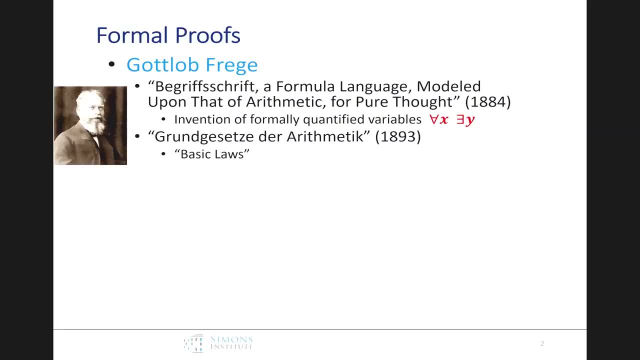 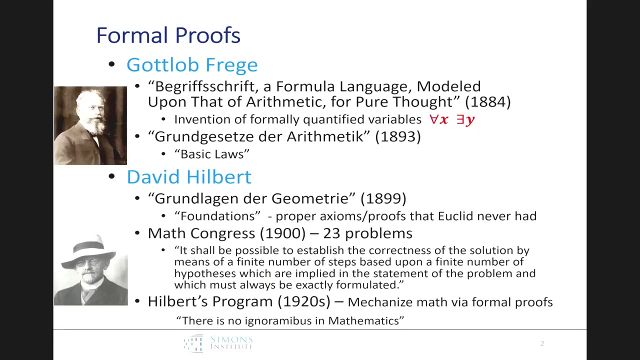 Variables and the quantifiers that we use now. Then, later in the 1890s, he spent a huge amount of work on a monumental what was intended to be two volume tome on the basic laws of arithmetic and how to develop everything from logical principles. The other, of course, is David Hilbert, who started- had already had a great career. 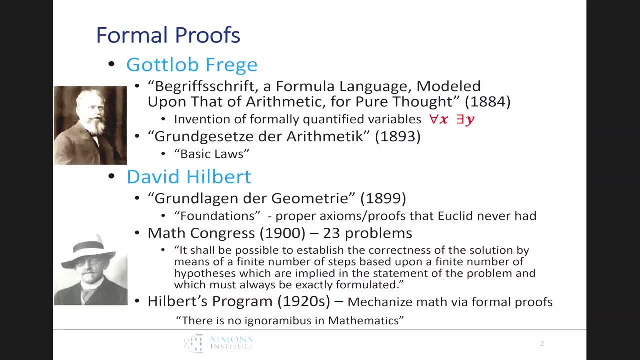 doing other aspects of mathematics but, starting in right at the turn of the 20th century, started to focus on questions about formal proof and formalizing mathematics, and his foundations of geometry in 1899 was at a level of formalism that even Euclid never had, and in his famous address at the math congress in 1900 where he set out his 23 problems, he very clearly 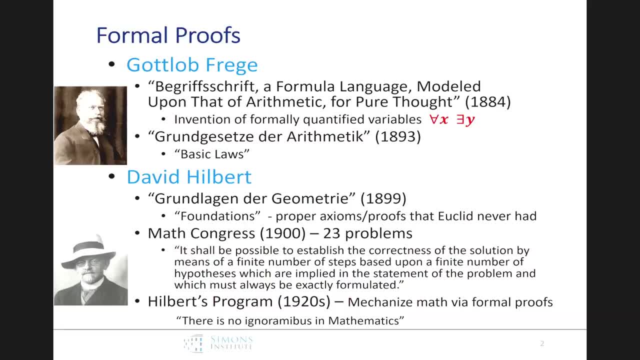 focused on the question of how to do things with formal procedures to solve all sorts of problems, and his program, which he proselytized a lot, especially in the 1920s, was really the program of mechanizing formal proof, and he's famous for the statement: there's no ignoramibus- we don't know in mathematics. so he's definitely was like. both of them were optimists and theorists. 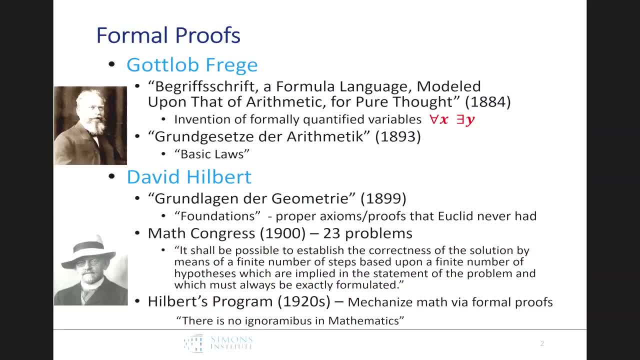 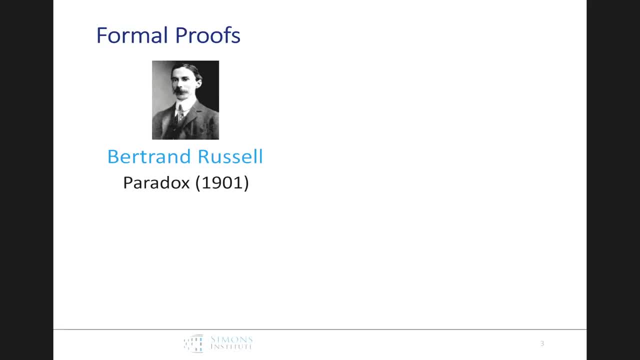 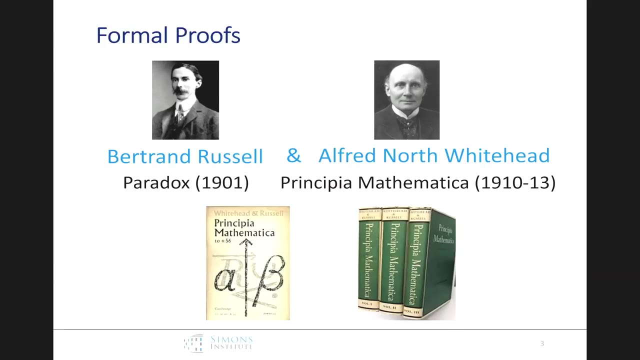 about formal proofs. Frege unfortunately got a little pessimistic when Bertrand Russell came along in 1901 and pointed out: you know this concept of the your system: you can talk about the set of all sets. well, there's an unfortunate paradox in that, and he, together with his advisor, Alfred North Whitehead, decided work the next 10 years trying to formalize all of mathematics- and you might be familiar with this volume. 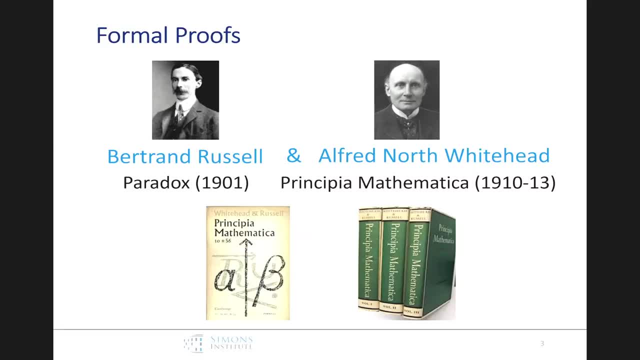 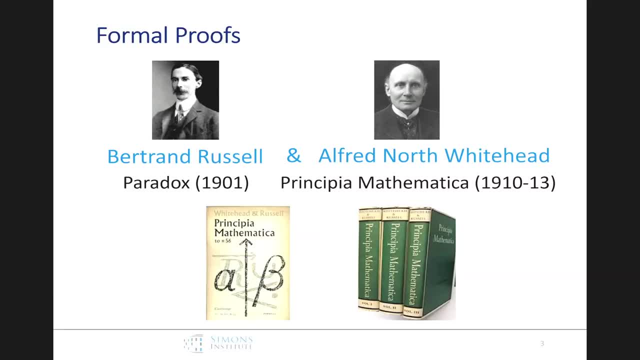 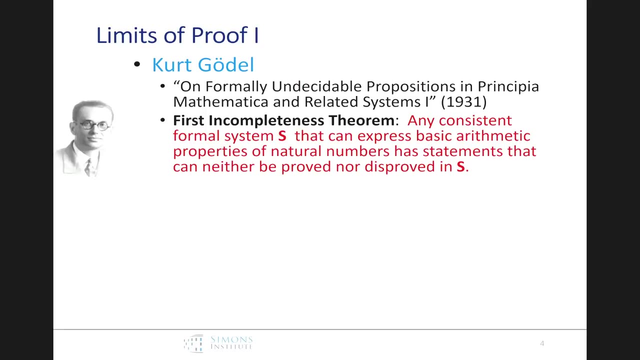 theory, but they really didn't get all that far in formalizing mathematics proper. and there was a reason for that. and that is the first limits to proof. and this good all, in his famous 1931 paper, showed that their project would be impossible if you wanted to express all the basic arithmetic properties of the natural numbers, any formal system you could come up with. that's 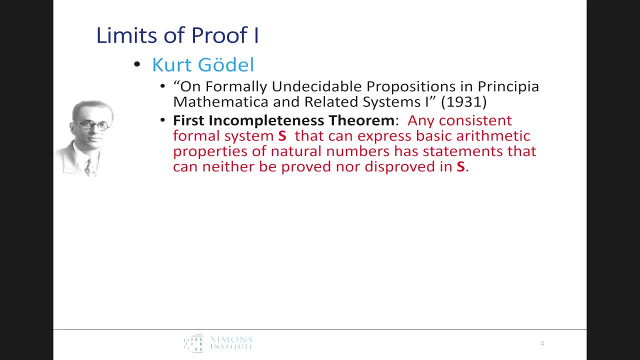 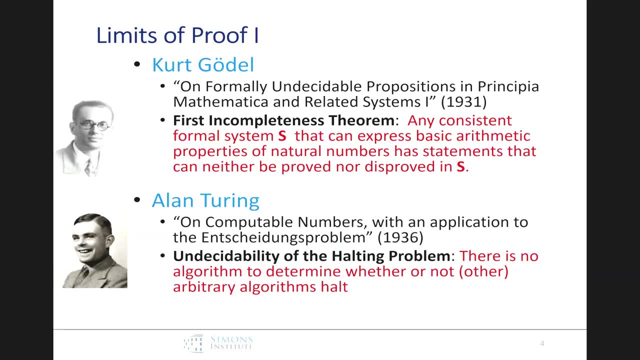 consistent would have statements that can either be proved or disproved. Turing came along and, inspired by Gödel and extending these ideas, showed that the halting problem is undecidable, in particular, that there's no algorithm to determine whether or not other arbitrary algorithms halt, and this in Scheidung's 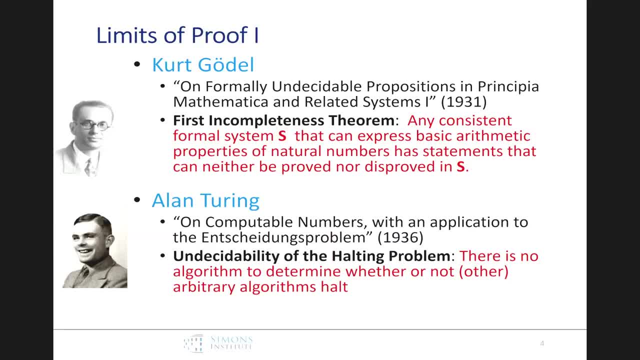 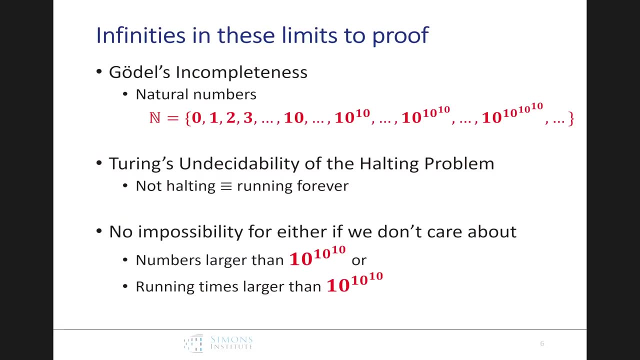 problem was actually one of Hilbert's problems. that was the inspiration for his work. of course, this doesn't mention proof, so we just tweak it. there's no system of proof that can prove whether or not arbitrary algorithms halt, so proofs very limited. well, there is an infinity in these limits to proof, so 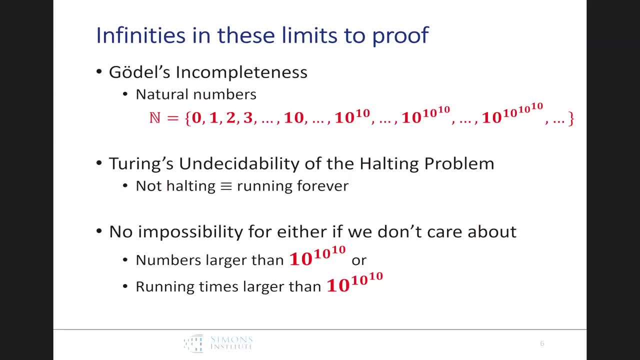 Gödel, incompleteness- we've got all of the natural numbers and Turing's undecidability of the halting problem. not halting means running forever arbitrarily large time bounds, so there's no impossibility result for either if, say, numbers larger than 10 to the 10 and the 10, or running time bounds. 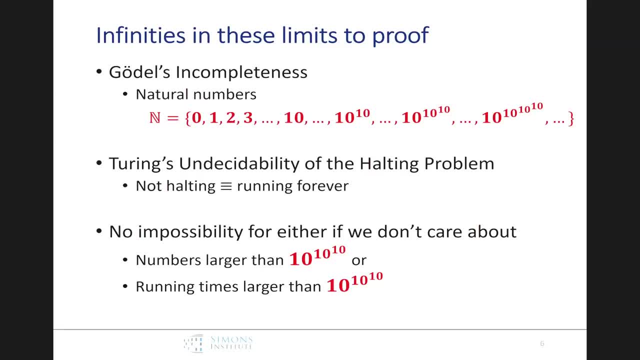 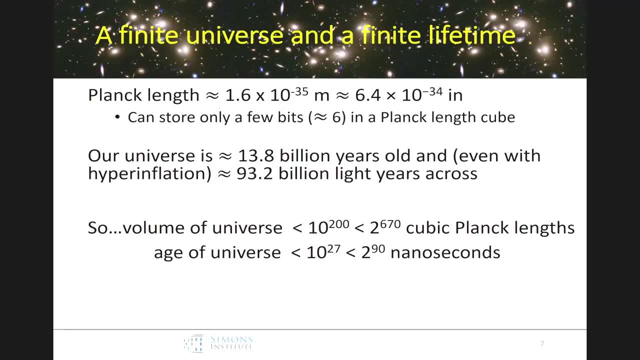 that big come into play. and well, we live in a finite universe with finite lifetime. so what's the? how can we think about the finiteness? well, a quantum theory tells us: Planck length is kind of the smallest unit unit of information. actually, if you take a Planck length cube, it's got six sides and you can. 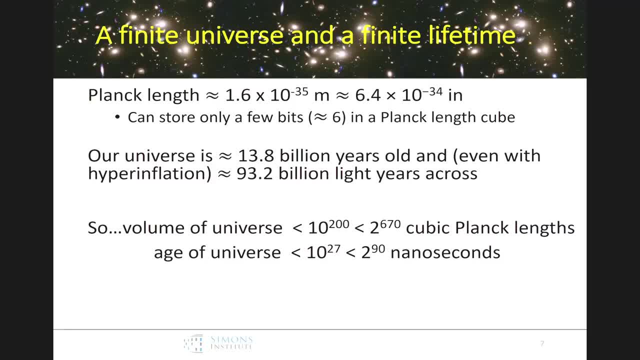 store about at most one bit per side, which is about six, and if you take the size of our universe and do it all out, the number of cubic Planck lengths is really not that big and the actual the time of a universe is really a very small if we, even if we, measured in. 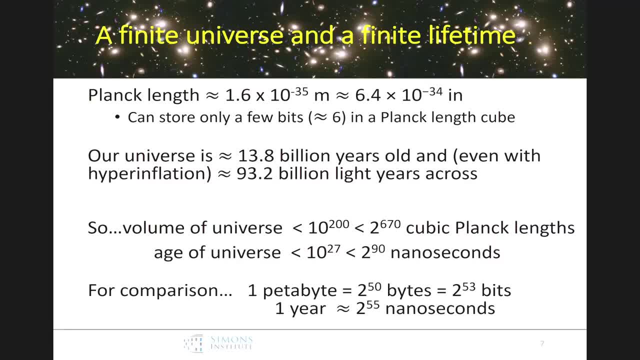 nanoseconds of the form of computers we do now, and so, by you know, just to compare these, we've got two to the 50th, which is sort of comparable there, and even a year of computer time is really not that far. in the exponent from the. 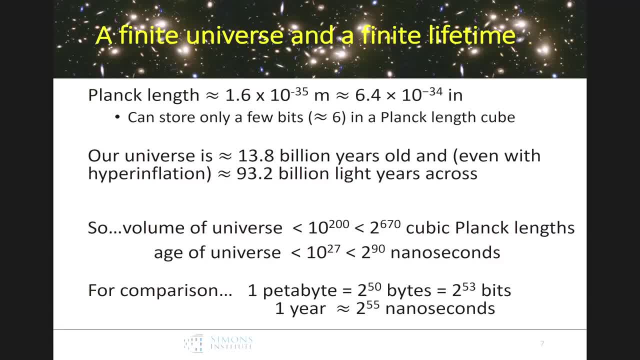 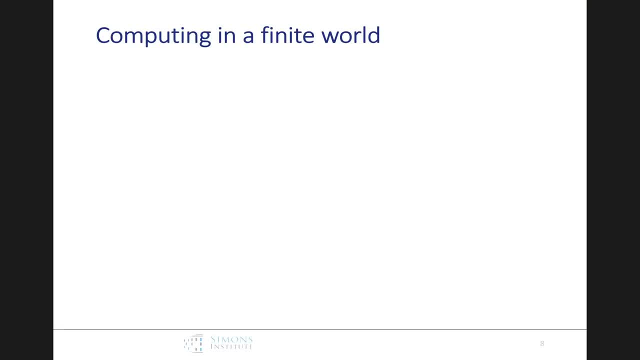 total life of the universe. so you know, maybe, maybe these infinite things aren't really a problem. and the first place is where this came up, as was in the notion of computing. we're computing in a finite world, so we're making. when people first did physical realizations of digital computers, they realized that efficiency. 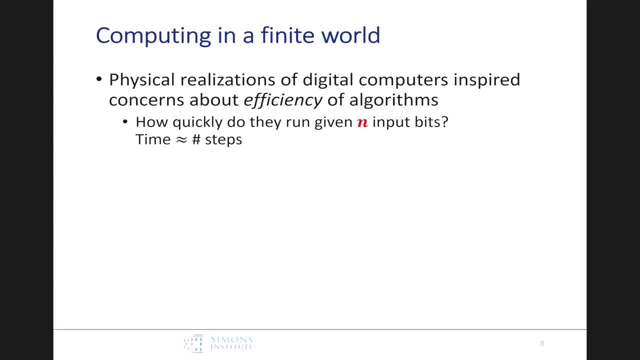 was important. in fact, von Neumann was famous for well known for going around, famous for it- and saying: well, we have to make sure that these algorithms run quickly. why was it? well, the computers would actually break down before the computation finished, and so on and so forth. you end up having a very complex 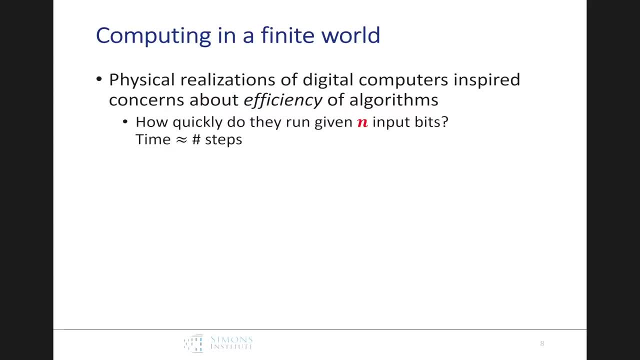 with the early computers. so that was the reason he was interested for a little bit more reliable now. but it was very quickly realized that there were good algorithms, algorithms that were bounded by number quantities, that are polynomial functions- the input size- and bad input, algorithms that are exponential and in 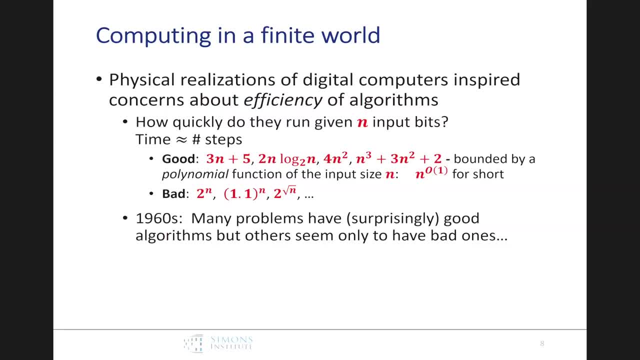 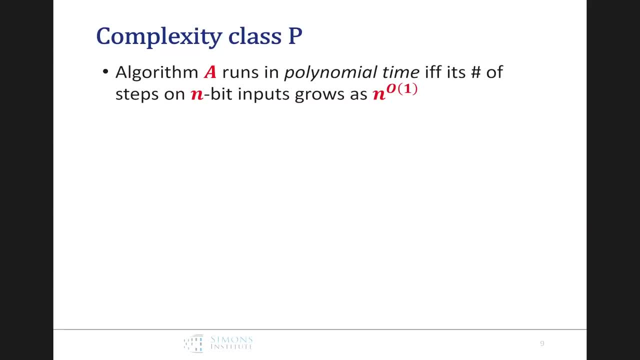 the 60s, people realized that many problems have often surprisingly good algorithms, but others only seem to have bad ones, and this motivated the definition of polynomial time, which probably is effectively due to Cobham. so it runs in polynomial time if its number of steps is grows as n to the order 1. 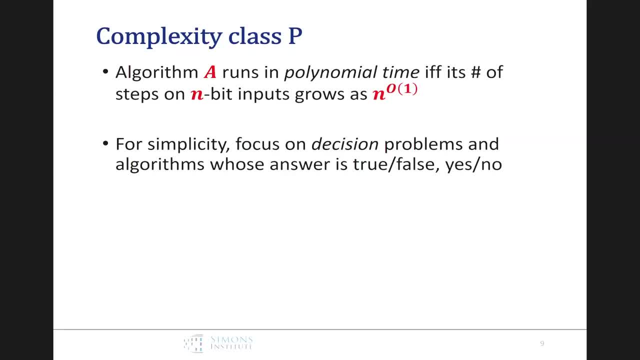 and for simplicity, we focus on decision problems. or the answer is just true, false, or yes, no, and define P to be the set of all decision problems with polynomial time algorithms. so that's the, the notion of computation, and the definition of the set of all decision problems with polynomial time algorithms. so that's the, the notion of computation. 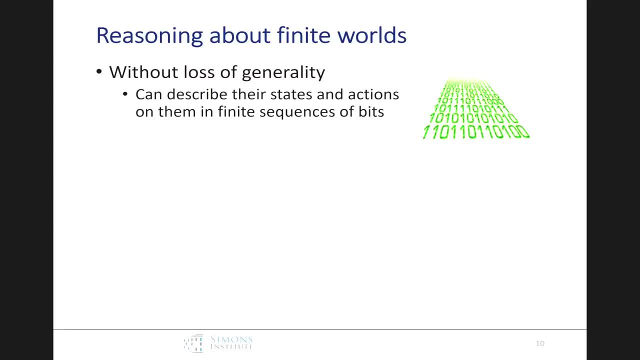 in a finite world? what about reasoning in a finite world? so, without loss of generality, we can represent any finite world, or and the states, the actions, whatever you want, by finite sequences of bits. I really don't want this going off to infinity, and there we can get to a much simpler logic than Frege or Hilbert. 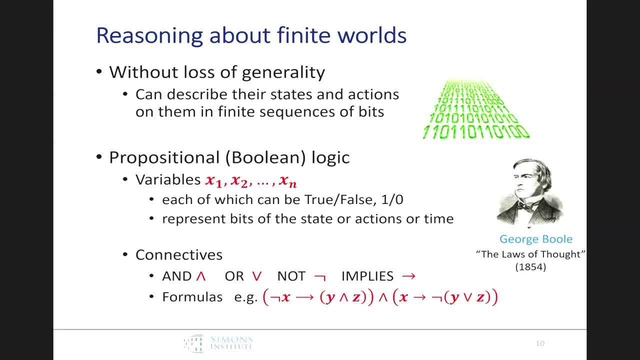 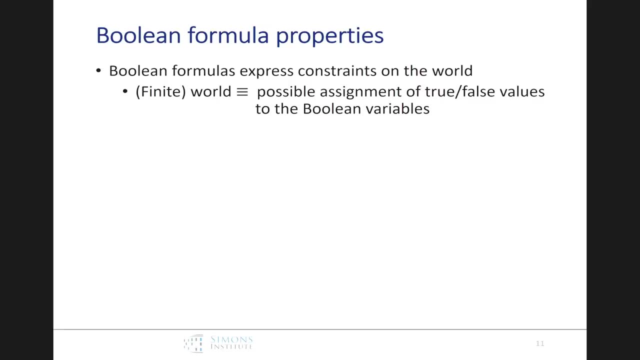 we're talking about, which is propositional logic, and going back to George Boole. so we've got Boolean variables and connectives, and or not, and implies. so what are the things we might want to understand about this logic? well, we want us the properties of Boolean formulas. these formulas express constraints that 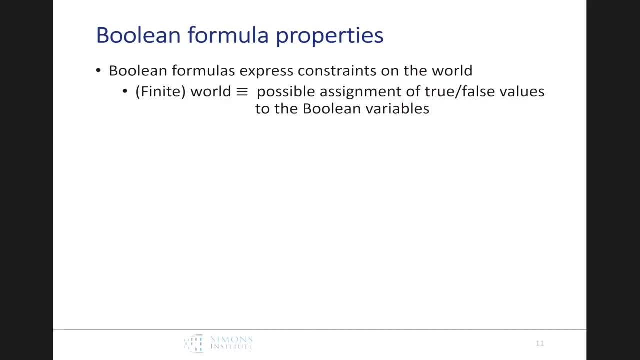 our world has to satisfy and the worlds are possible assignments of true, false values to these Boolean variables. so we've got properties like satisfiability. a formula is satisfiable true if in some worlds, tautology it's always true, and unsatisfiable if it's. 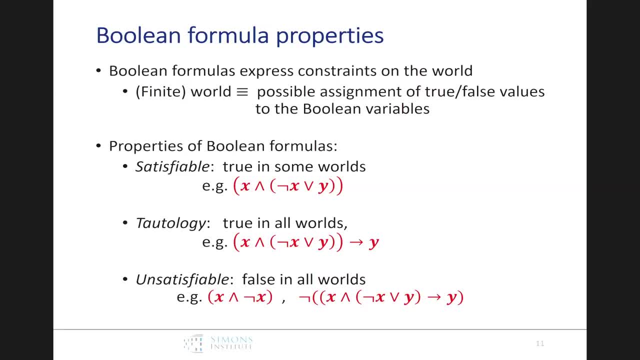 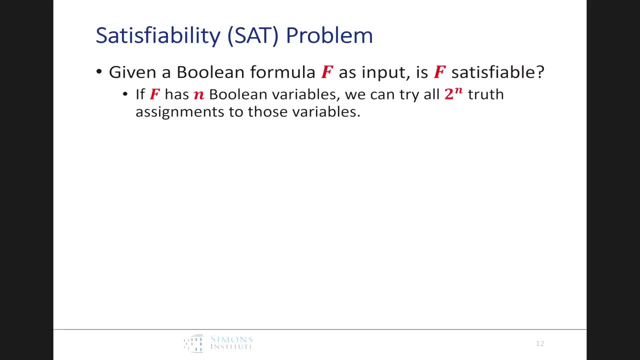 always false in all possible words. so here's a simple one, and it's nice you can go back and forth between tautology and unsatisfiability just by sticking knots in front. okay, so the first of these problems that get tackled is the problem of satisfiability. you know this audience probably. probably we're gonna. 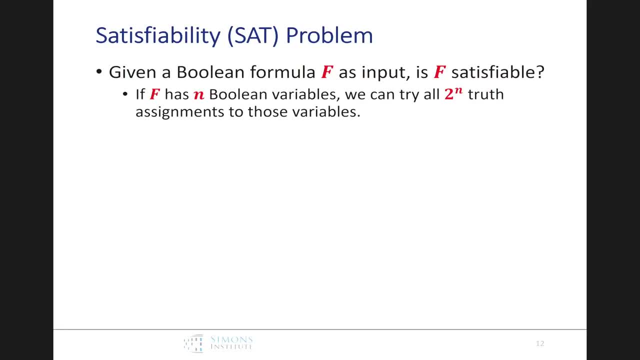 be a little bored for the next couple minutes. but so if it has boolean variables we can try all assignments. so the question is: is this problem of deciding whether a formula is satisfiable, is it polynomial time? of course it's open, but there is this related problem where we have a 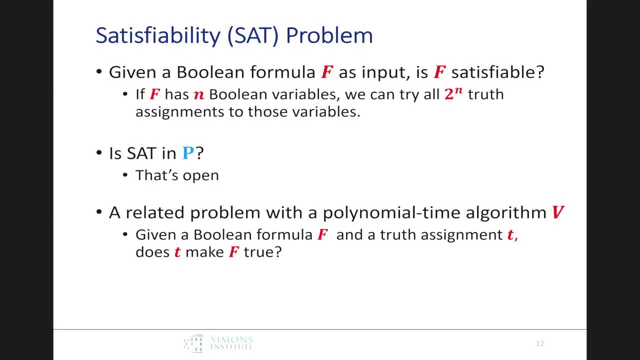 polynomial time algorithm, which is given a boolean formula and a truth assignment to it, does that truth assignment make the formula true? so there we do have some polynomial time task and a formula is sat if, and only if, there exists some T. that makes it true, which means there exists some T. 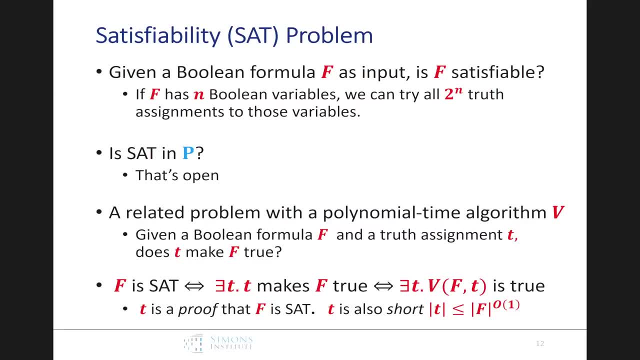 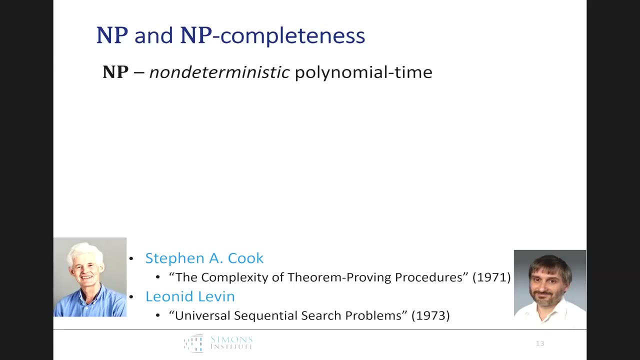 such as a verification algorithm that's checking whether T set makes it true says yes. so T is a proof that f is sat and the other piece about it is: it's also very short. in fact it's linear in the size of the input. so of course, cook and levin famously generalized this notion of 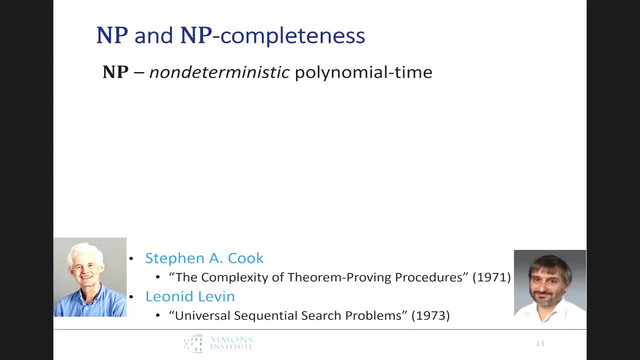 Havin something that's paner specific rather than numerical keyカ��는 and could never compare it to anything like k Agora. that's easy to check, like checking, like the satisfying assignment. assignment satisfies the formula makes it true with non deterministic polynomial time. so we 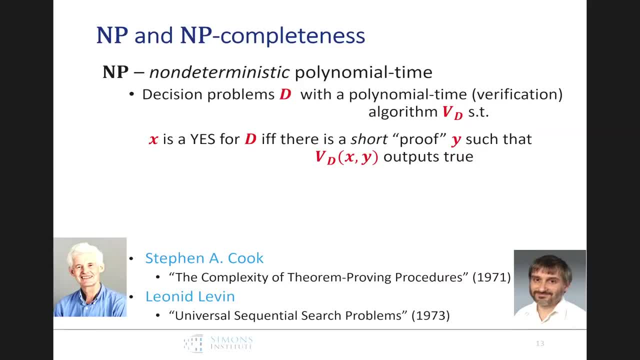 can write it. I'm going to write it in a formal way. so these are decision problems that have a polynomial time associated verification algorithm, such that a string X is a yes for the decision problem if, and only if, there's a short proof- why? such that this verifier checks out and says: why does? 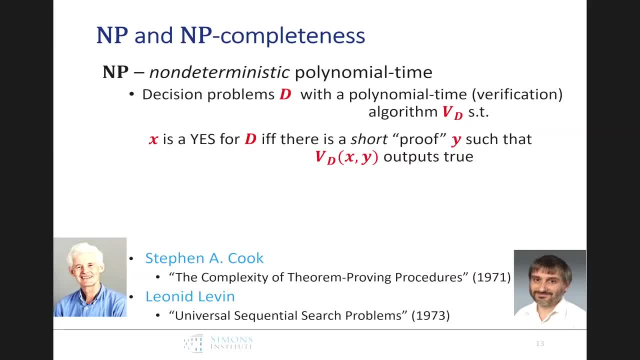 prove that X is is, is is a yes for that problem. and by short we mean polynomial. so of course SAT is NP complete. that's the big result of both cookin and Levin, on opposite sides of the Iron Curtain, which means that if SAT isn't P, then P. 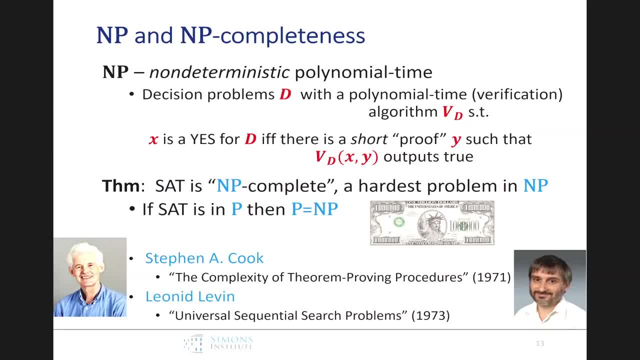 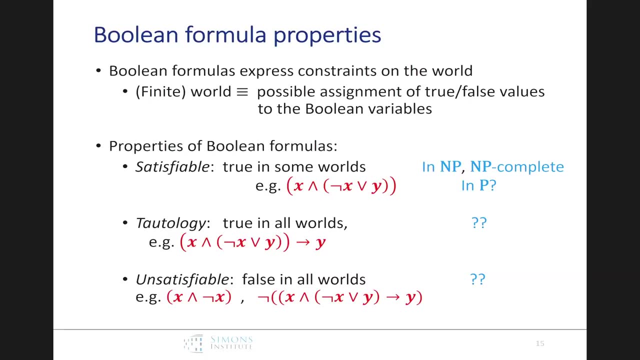 equals NP and figure that out, and the clay Institute will give you some, some data bills of that form. so a million dollars, uh, so boolean formulas. so these are the same problems we we had before. so we, we know, really have a decent understanding of satisfiability. obviously, big open questions about it. but what about? 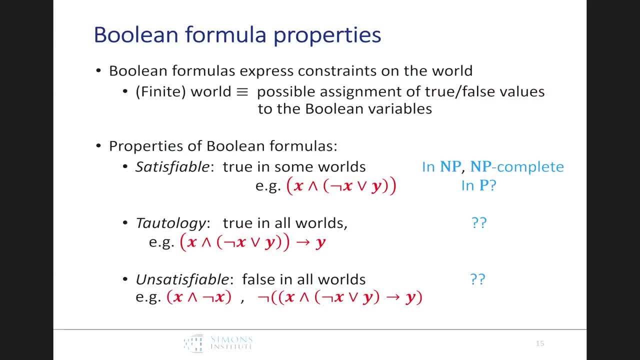 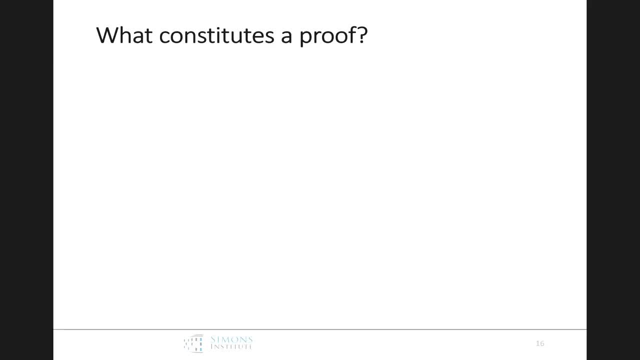 tautology or unsatisfiability. so for this we need to think about what constitutes a proof of tautology or satisfiability. well, here's the conventional textbook proofs. so we've got some axioms like excluded middle inference, rules like modus ponens, and a proof is a sequence of lines, each which follows either from: 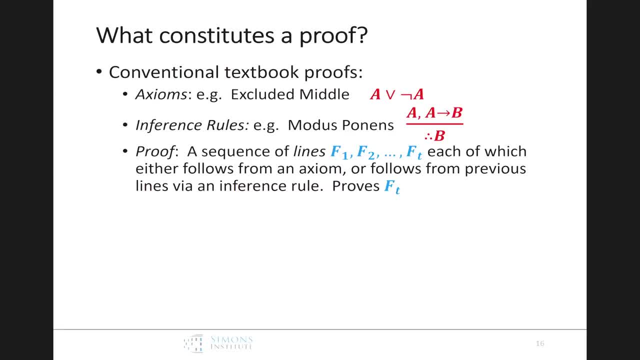 an axiom or from an inference rule, and the last thing you've got is the thing you're proving so. but another thing that's also a proof would be truth tables. these are also proofs. they're very easy to check locally. you can just check how each more complicated formula depends on the previous simple ones, and 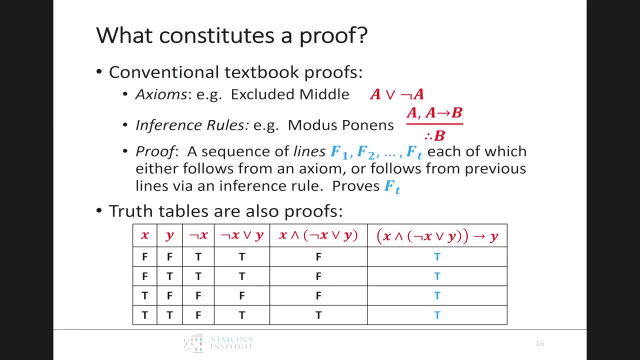 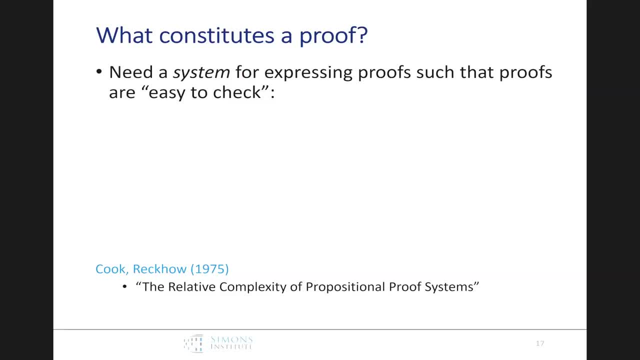 then you just check the final line, so that is a proof as well, and cook and Recco realize that there's something more general going on here. we need a system for expressing proofs so proofs are easy to check, and that's the key property of both the truth tables and these, these inference systems. so we think 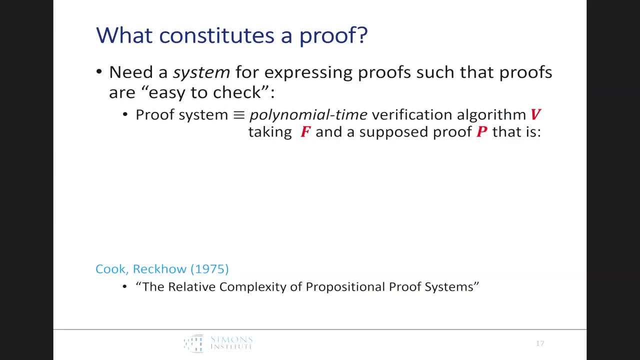 about it is this polynomial time verification algorithm that's going to check the proof, taking a formula in its supposed proof that sound it outputs true? if it does, then you've got something that say a tautology, or unsatisfiability or unsatisfiable, and it's complete for every tautology there. 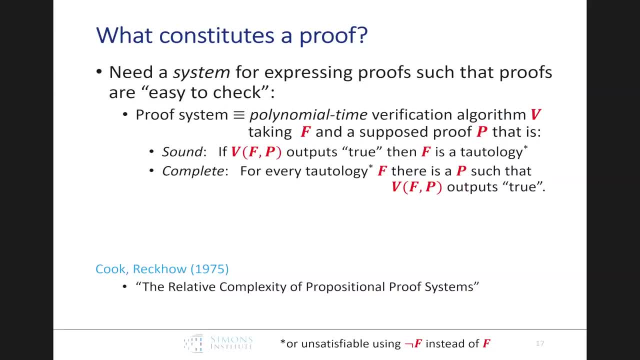 is a proof such that the verifier likes it, the verifier checks it out. so this is very much like the definition of a proof of truth and it's very much like the definition of NP. but there's one critical difference: there's no requirement that this proof P be short. okay, so that's the sole. 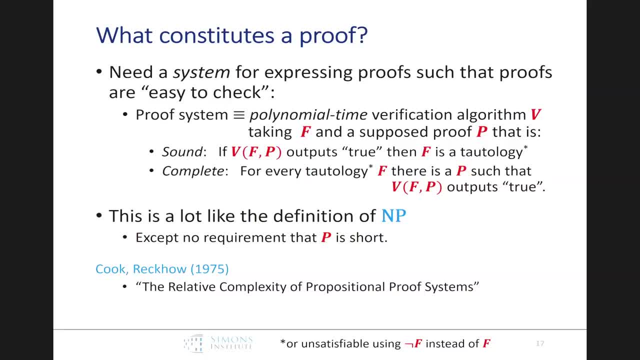 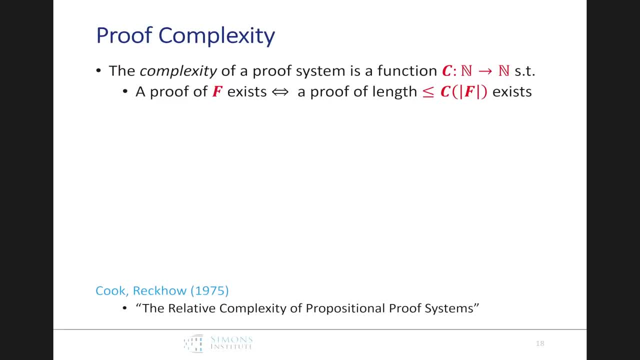 difference from the definition of NP. this easy to check, this- having the sufficient verifier is is the key piece. so so the once we have this, we need a notion of complexity. truth tables aren't as good as as these other inference systems, but they're not as good as these other inference systems, but they're not. 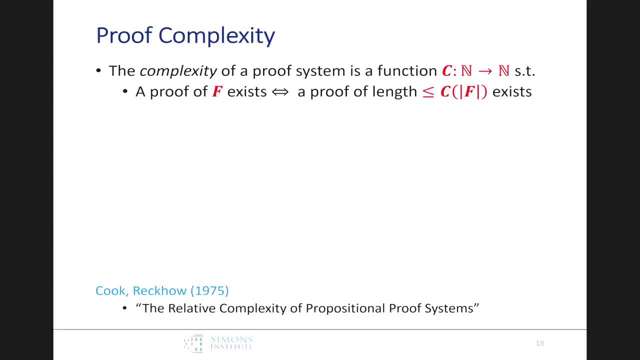 as good as these other inference systems, but they're not as good as these other practice are asking for writing down proofs. so the complexity of a proof system will exactly captured this question of: well, how big does the proof actually have to be? so C of F, it's a. 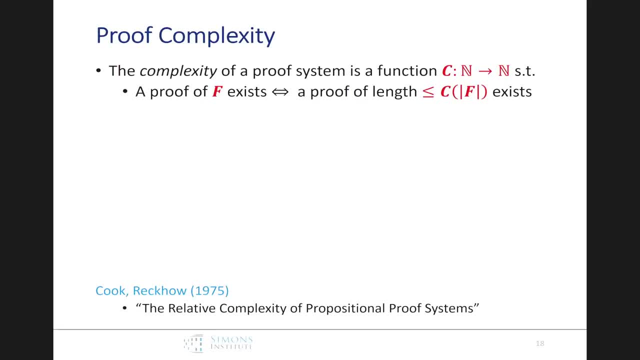 it's a. it's a numerical bounder, numerical function that tells you, given how big your formula is, how big the proof has to be. so truth tables have complexity, at least two to the end. you just need two to the end rows to write them down if they're end variables in your formula. now 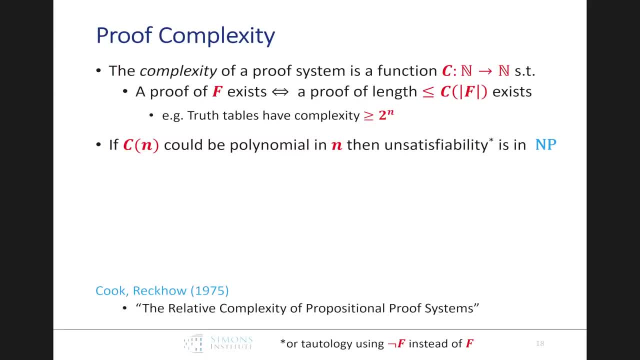 C of n. so if we could show, find a system where C of n is polynomial in n, then we have a proof of tautology or unsatisfiability being an NP, because this would be that one extra missing condition about the shortness of proof. 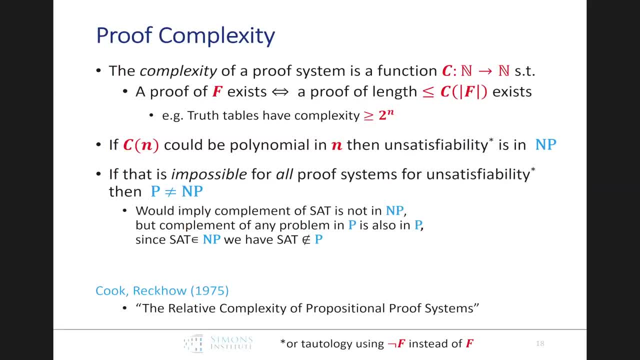 On the other hand, if we can show that it's impossible for all proof systems for unsatisfiability, it's impossible for this to be polynomial in n for all proofs of unsatisfiability, then we would conclude that P is not equal NP. And here's the quick idea. well, unsatisfiability is the complement of SAT. 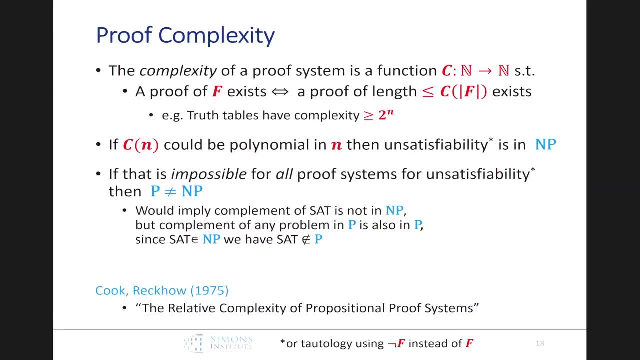 so we'd say that that's not in NP. but if we were in P, so the complement of any problem in P is also in P. and since SAT is in NP, its complement, if it were also in P, its complement, better be so. SAT is not in NP, So 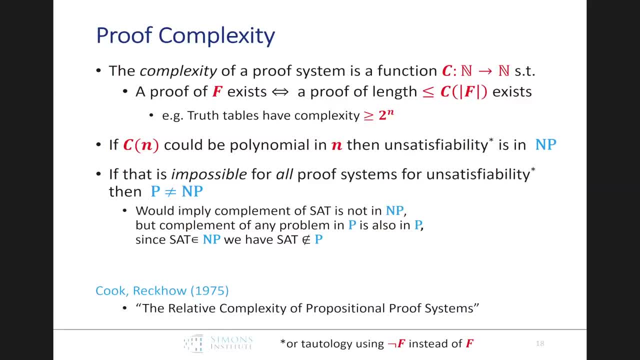 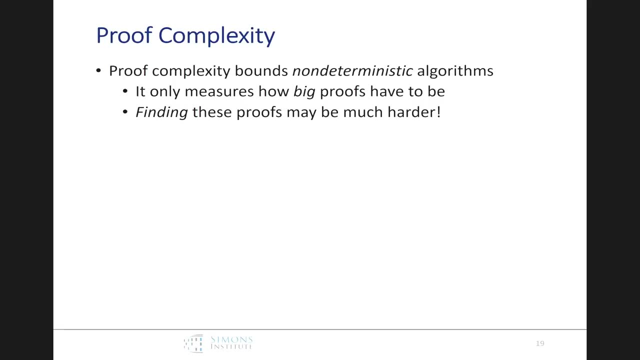 alright. so this question of how big proofs are is really the fundamental question of proof complexity, and it's a very interesting question from the point of view of of what it's trying to say, because proof complexity just doesn't, doesn't just bound. what deterministic algorithms can do, how long they'll take. 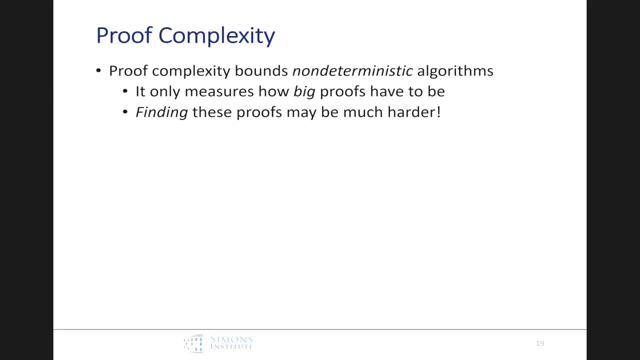 it bounds non-deterministic algorithms as well, So it only measures how big proofs have to be, how many symbols it takes to write them down. it doesn't say anything about how complicated it is to find them, and in general, the search problem finding a proof might be as 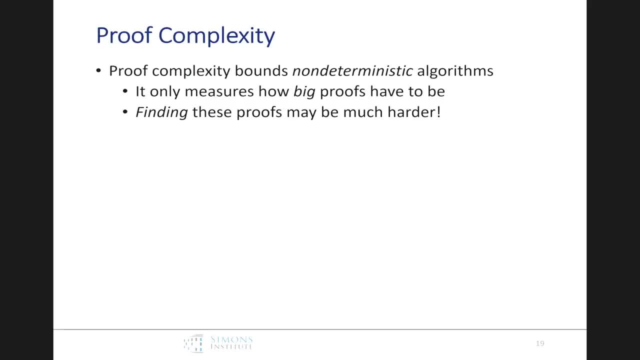 might be require some form of exhaustive search, so finding the proofs might be much harder than just writing them down. However, you might think: well, proof systems, we came up with a couple. there are actually many, many proof systems. one can come up with any deterministic algorithm for SAT. 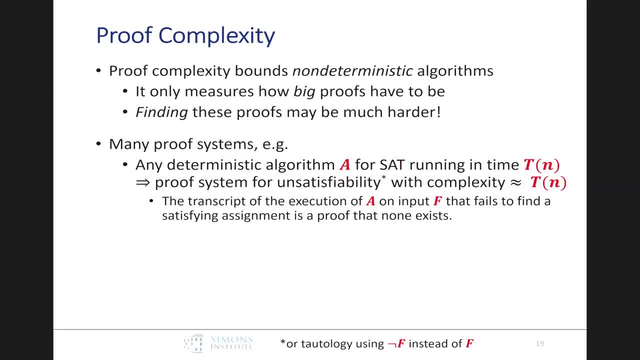 with a running time. t of n yields a proof system for unsatisfiability with complexity roughly like t of n and the basic idea is: if you've got some unsatisfiable formula you want to prove it's unsatisfiable, just run the algorithm and write down the transcript of all the states you've been through and 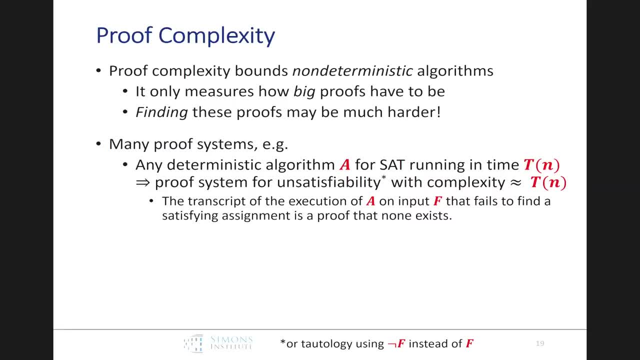 that is a proof that no satisfying assignment exists. if you had a deterministic algorithm for SAT. So that's one way we can come up with a proof system, And this method actually does relate to some things in practice, as we'll see. The proof complexity program, if they could say that is. 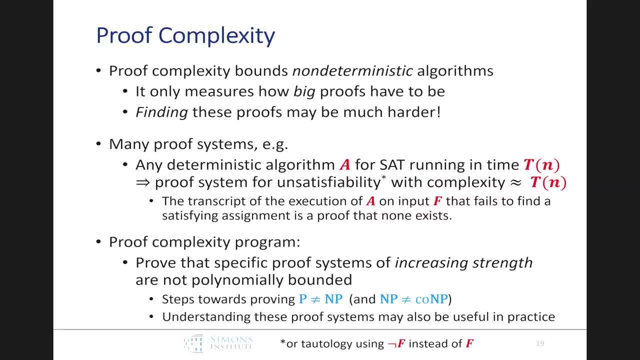 to prove that specific systems of increasing strength are not polynomially bounded. So so one of the reasons why you might want to do this is as steps towards proving p not equal np. You don't have to do this. It would actually prove something stronger potentially, that np is different from co-np. 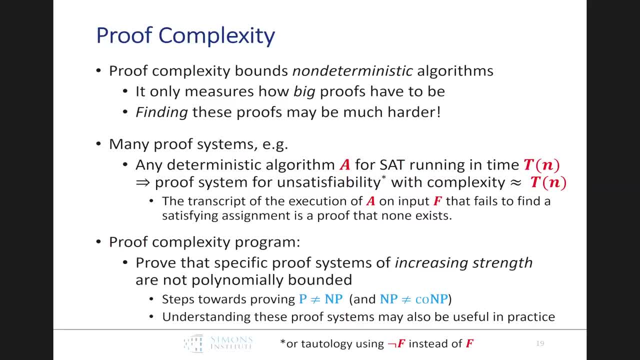 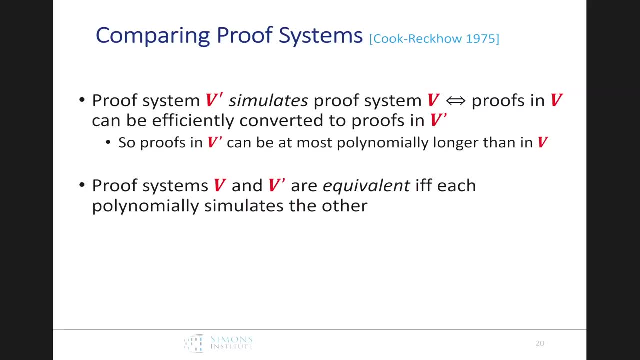 I won't go through the definitions, But the other thing is that understanding these proof systems may also be relevant and useful in practice. Okay So, but how do we compare strength of proof systems? So Cook and Recco said: well, if one proof system simulates another. 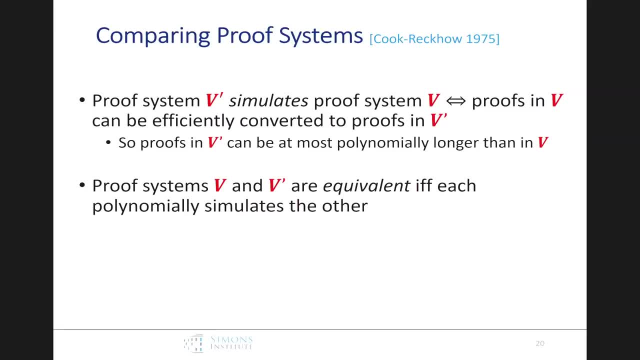 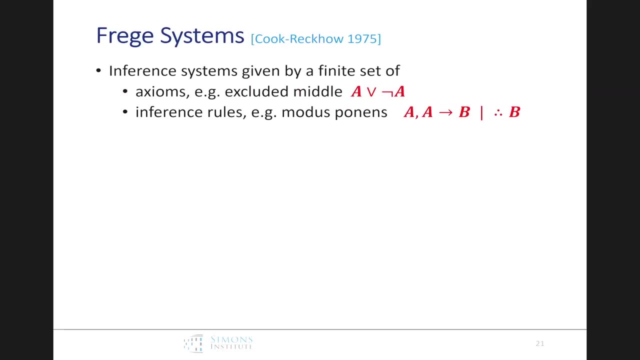 if proofs in one can be efficiently converted to proofs in the other. So it tells you that proofs in that one can be at most polynomial than proofs in the original system. And proof systems are equivalent if, and only if, they simulate each other. And one of the first systems that class of systems that Cook and were analyzed by Cook 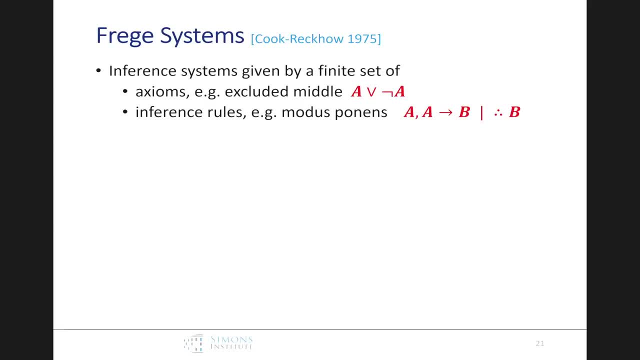 and Recco, which they called Frege systems and are largely known elsewhere before this as Hilbert systems, even though Frege had essentially defined them much earlier, but Hilbert was a big popularizer of them. These are inference systems that are given, just like the ones we've seen, a finite set. 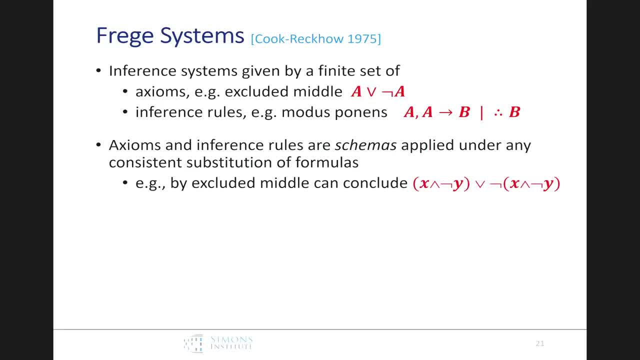 of axioms and inference rules, And the axioms and inference rules are actually used as schemas where you get to substitute consistently into the formulas. So for example, given this axiom a or not a, we can plug in x and y And say we can automatically conclude that this line is true. 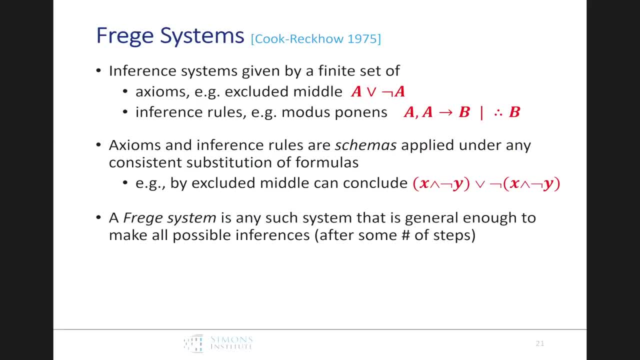 Now a Frege system is any such inference system that is general enough to make all possible inferences after some number of steps might take you a while, And what Cook and Recco proved is that all of these Frege systems, no matter how you define, 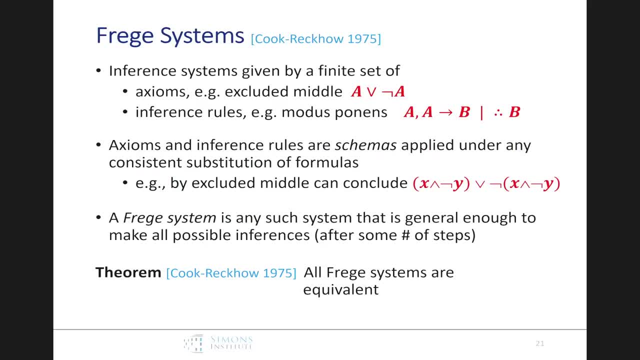 them are all equivalent to each other. They can be. the proofs from one can be converted to proofs And the other and it's actually not too difficult to prove. Now, Frege systems and proof systems in general deal with arbitrary Boolean formulas as input. 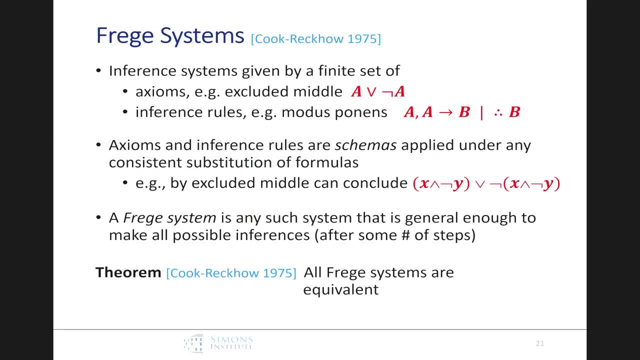 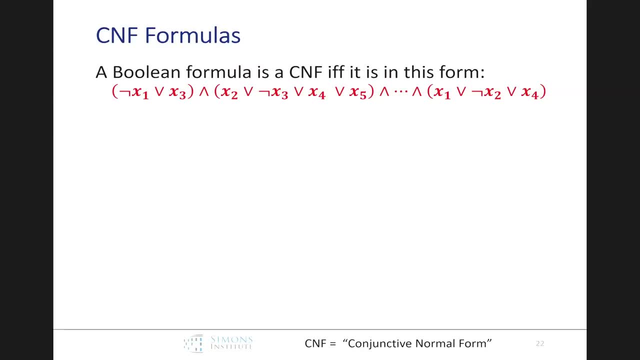 And it would be nice to have something, a simpler version of input to deal with And here's a nice form that's very convenient for as input to these proof systems. So a Boolean formula is a. CNF stands for conjunctive normal form. 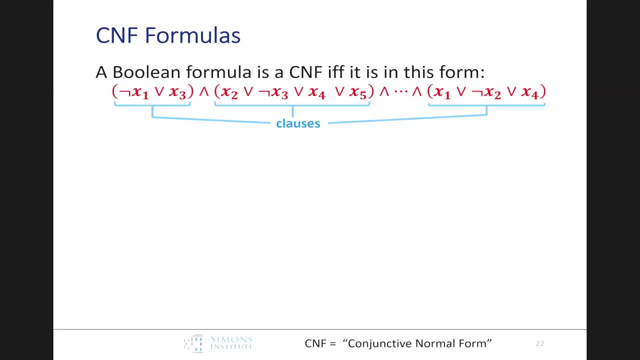 If it's of the following form. we've got a bunch of it's an and of a bunch of clauses, Each of which is an, or of a bunch of literals, Each of which is a variable or it's negation. So this is a nice, flat, simple type representation that happens to be very good on to represent. 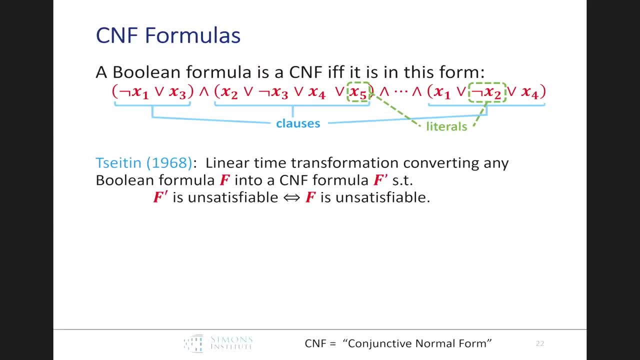 on computers and to work with. And Seiden in 68 showed that there's a linear time transformation That will convert any Boolean formula F into a CNF formula that has the same satisfiability properties. So we might as well just work with that CNF formula. 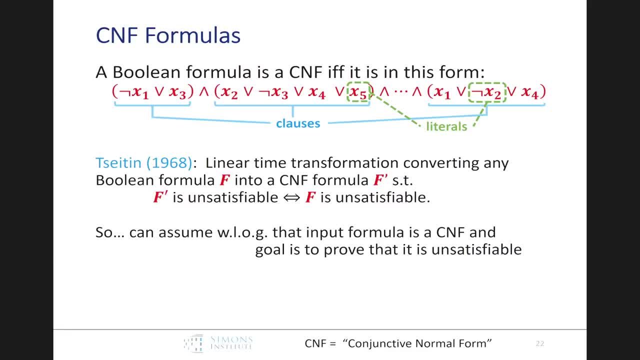 So we can assume without loss of generality that our input is a CNF formula, because we could just quickly do a conversion of the sort that he suggested. And this is of course part of the standard proof that three SAT is NP. complete and just for completeness. 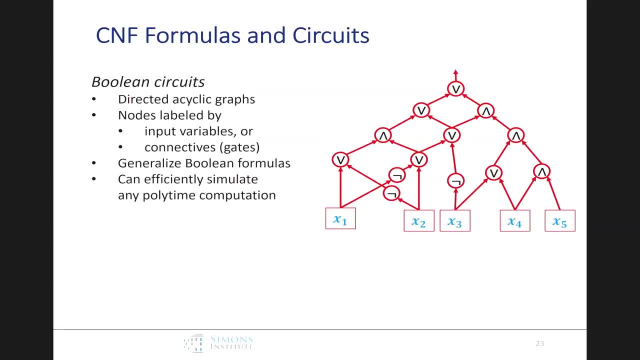 I'll describe the construction. So in general it works for arbitrary Boolean circuits, And these are graphs which have variables as their input and these connectives as gates, And the main difference from Boolean formulas is that in Boolean formulas there will only be one output edge from each gate, whereas here you might have multiple inputs. 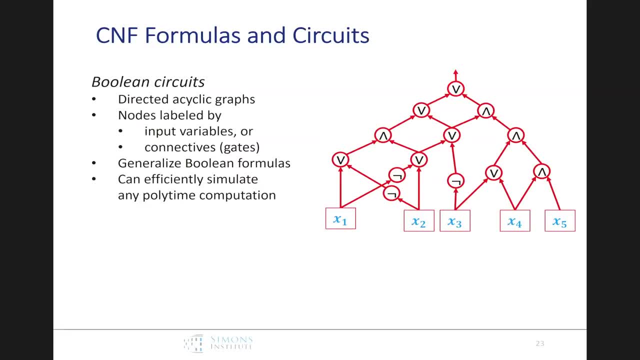 And, of course, and these can in fact efficiently simulate any polytime computation And The Seiden transformation. is is nice. you actually add some extra variables, one for each of the gates. Okay, That's going to express the value of the gate. And then we add clauses one, an, and of clauses, one, clause to say that each internal gate 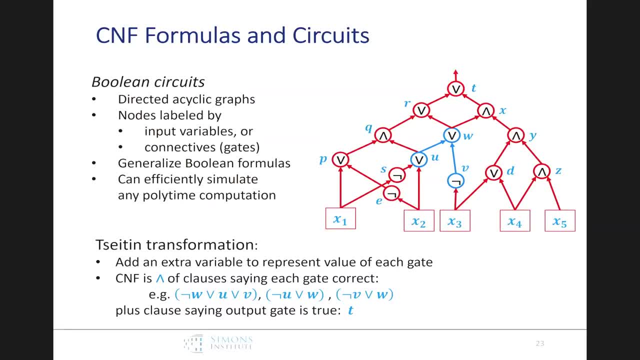 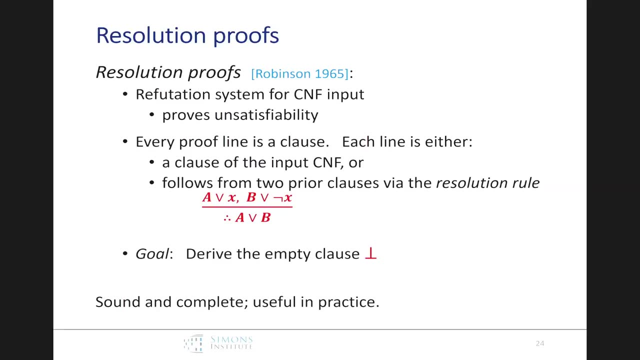 is computed correctly and a plus a clause saying that the output gate is true. Okay, so we've got CNF formulas. inputs are dealing with clauses. wanted to a proof system that just deals with clauses And that's resolution proofs. this is a reputation system for CNF input. every proof line is a. 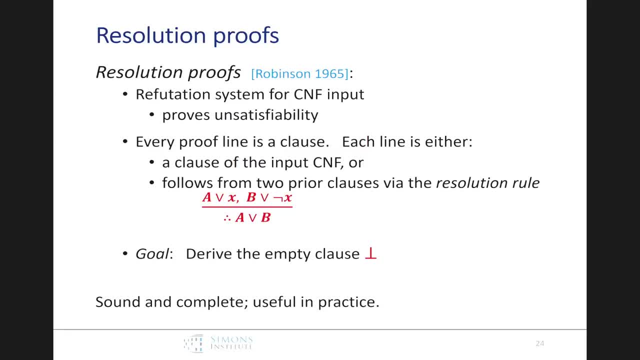 clause. each line is either a clause of the input or follows from two. it's got one inference rule, one inference rule only. we take two clauses and they have variables of opposite signs than the or of the remaining variables. has to be true, because no assignment can make. 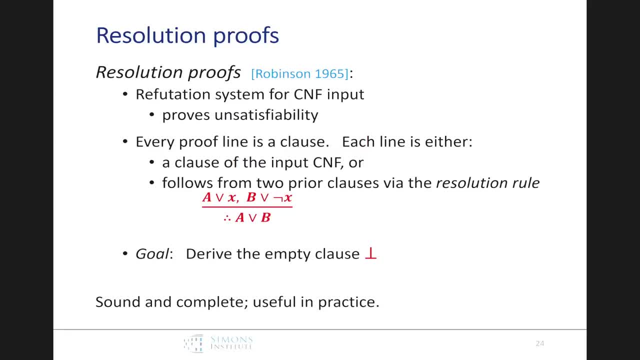 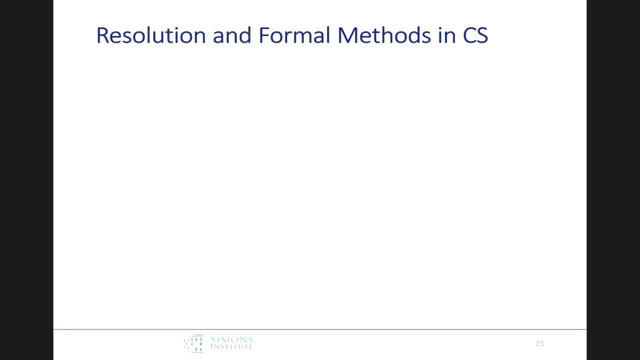 both, the both of two X can make both of these true and the goal is to derive the empty clause Okay, Which can't be made true because there are no variables in it to make it true. This is sound and complete for four clauses and it's incredibly useful in practice. 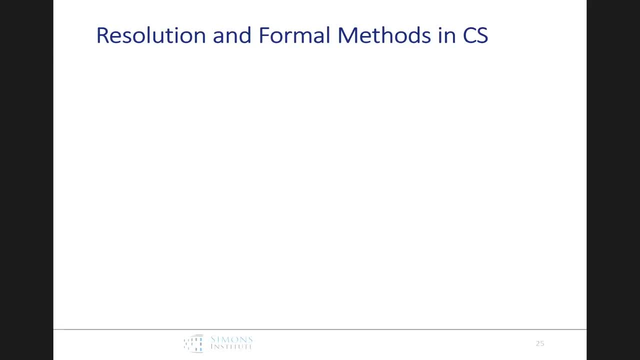 So Resolution has a strong connection to formal methods in CS and if since, I would say about 2000, formal methods for analyzing software and hardware using SAT solvers has just really revolutionized the field of, of of analysis for for computing, and the general idea is: 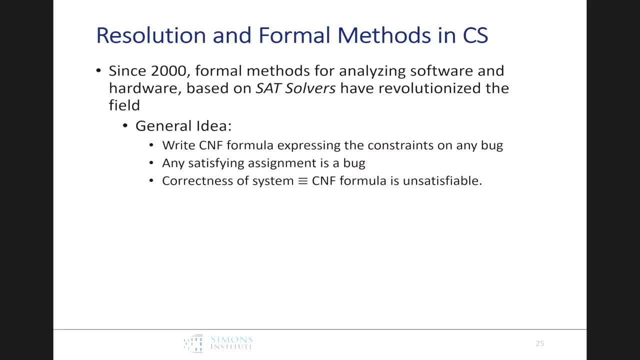 you write a CNF formula expressing the constraints that any bug has to satisfy. So any satisfying assignment is a bug. So the correctness of a system is equivalent to showing that the CNF formula is unsatisfiable. and the fact that we can do write these even for circuits is is extremely convenient. 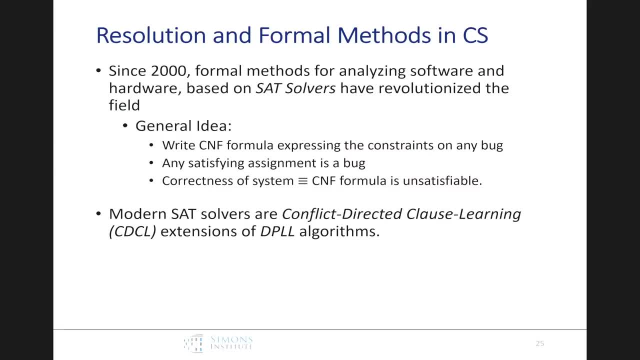 Now Modern Solvers are what are called conflict directed clause learning or CDCL, extensions of DPL algorithms, And they're extremely successful CDCL solvers. I mean they work well on CNF formulas with tens to hundreds of thousands of variables, millions of clauses, even though we know that 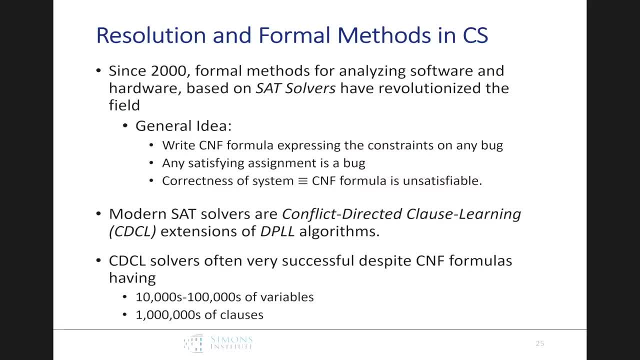 SAT is empty, complete. That doesn't actually mean that they always work- And There are. There are a number of ways that people were initially were trying to solve problems using these solvers and they ran into some problems that actually turned out to have been previously. 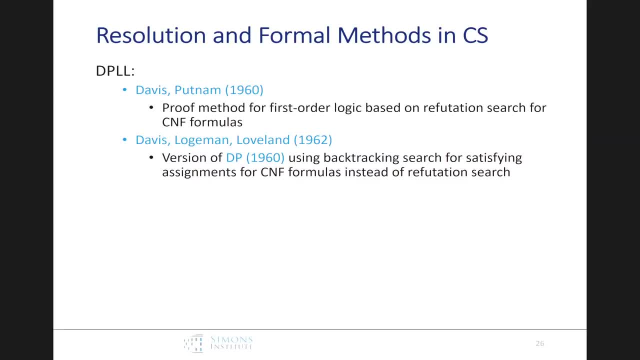 Oh sorry, let me back up. So let me explain a little bit about these solvers: CDCL and DPL. So DPL comes from the name of two papers by Davis, Putnam, Logeman and Loveland. One of them is called DPL. 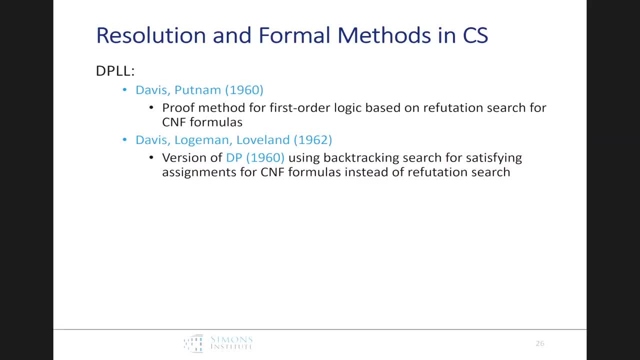 And the other one is called DPL. The first doesn't have anything to do with the DPL algorithm but showed how you could translate first order logic into refutation search for CNF formulas. The later paper is what introduced the backtracking search for satisfying assignments. that really. 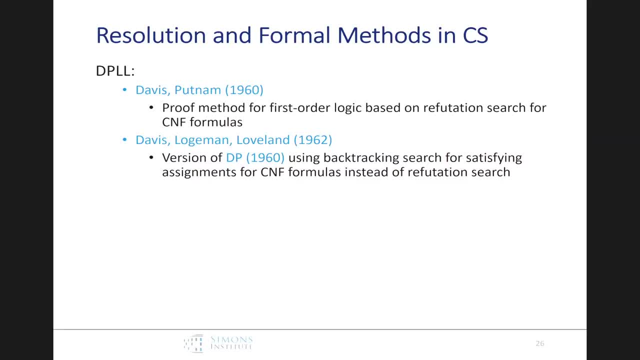 and plug it into the approach of the first paper. that really is the basis of the modern algorithms. but just to keep various people happy, the P is kept in the middle. So So, So, So, theIMP. So the, it's not hard to show. 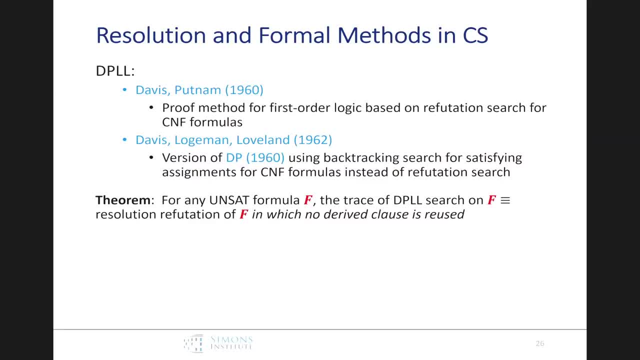 It's, I couldn't even think of what a references it's like. folklore is that if you've got an unset formula and run DPL search on it and it fails, that trace thing becomes a resolution refutation of the original formula but of a special form. when you derive a clause, you 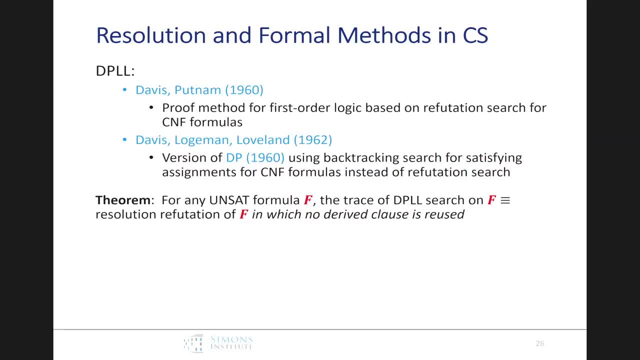 don't get to reuse it. So you derive a clause and you want to use it again, you have to derive it again. So that's a very restricted form of resolution. proof CDCL covers these are extensions beginning late 90s- 2000s, which primarily the new thing. 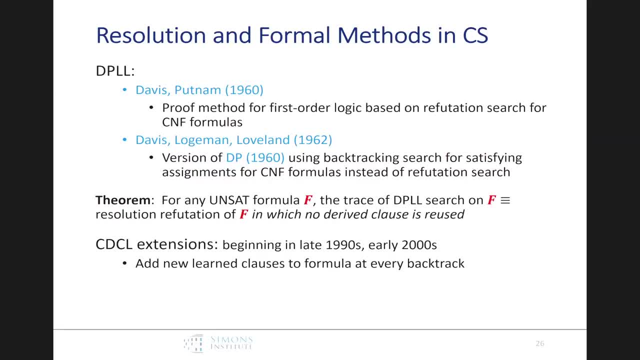 was adding new learned clauses to the formula at every backtrack and there are also things like restarts and a lot of other tricks, but you can also show that resolution covers. you know the traces of these things when they fail to find a satisfying assignment. 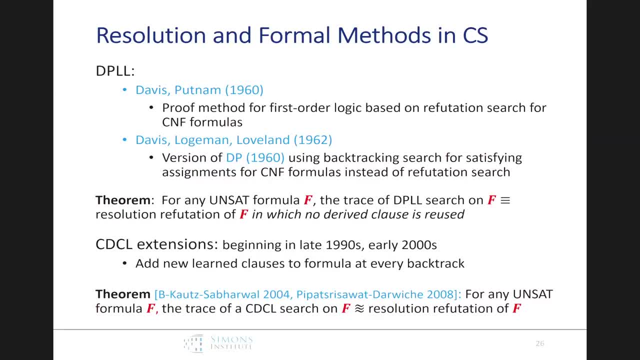 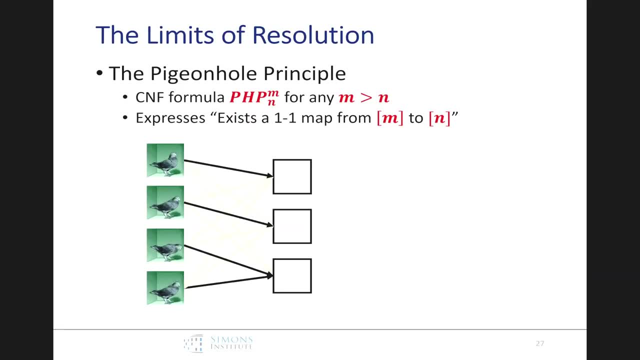 are actually resolution refutations of the formula. So resolution really does capture what these SAT solvers are doing And, as I was mentioning earlier, there are limits to resolution. So one of the limits is the famous pigeonhole principle. So these four pigeons want to go to these pigeonholes for the night, and the problem? 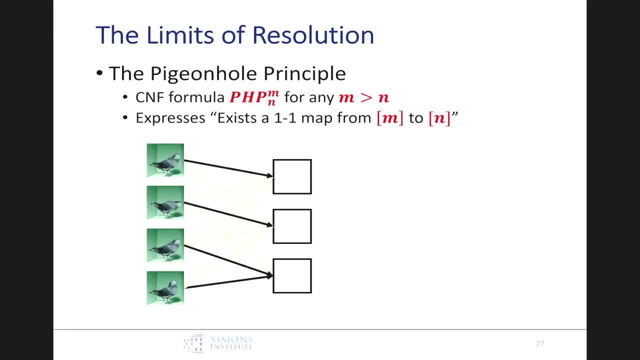 is that two of them- you know at least two of them- are going to be unhappy because they land in the same pigeonhole. So how do we express this in Boolean logic? Well, we have a variable for each of these possible edges. xij says that pigeon i maps. 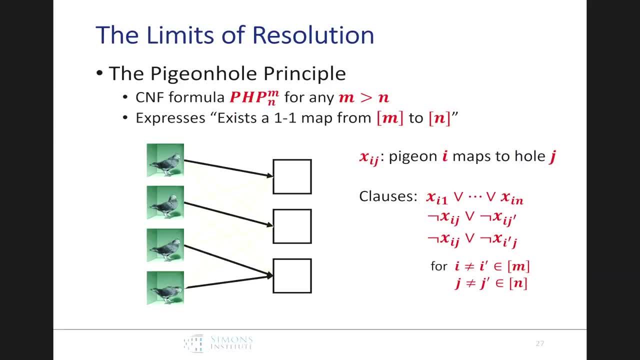 to hole j. We have clauses that say so. this says every pigeon is mapped somewhere. this says it's only mapped to one place and this says every hole gets at most. these say every hole gets at most one pigeon And this is unsatisfiable by the pigeonhole principle. 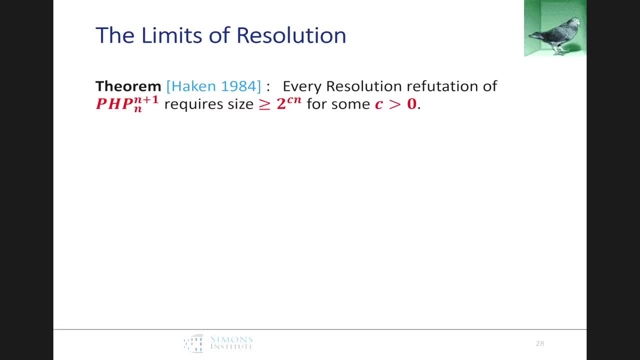 Well, Hawkins showed in 1984 that every resolution refutation of the pigeonhole principle requires exponential size. Now remember: exponential n doesn't have to be too big before this is larger than the number of symbols you can represent in the universe. 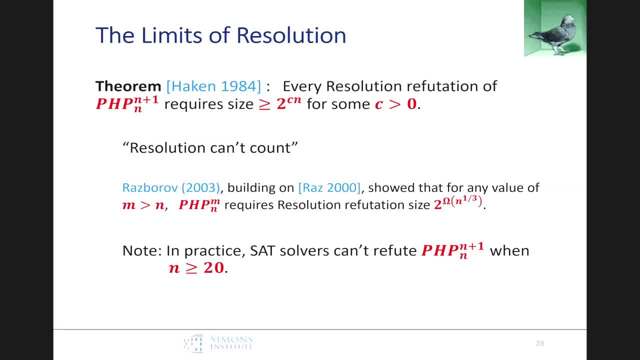 And so resolution can't count. And then later Resborov actually showed that it doesn't matter how many extra pigeons you have. resolution still can't figure it out, And in practice this really is an issue. SAT solvers can't refute the pigeonhole principle when it's like roughly 20 variables, or maybe. 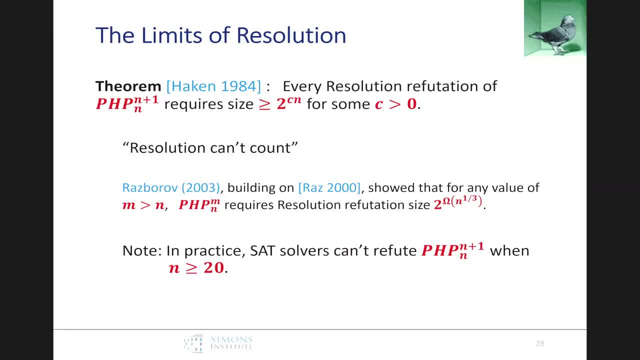 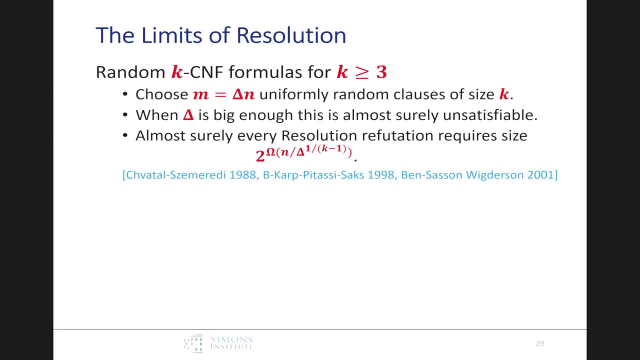 a little bit more than that. So, even though they can handle thousands of variables, this is only a few hundred variables and they get stuck. Another class of formulas where these solvers have major problems are random formulas. So take a random KCNF formula. 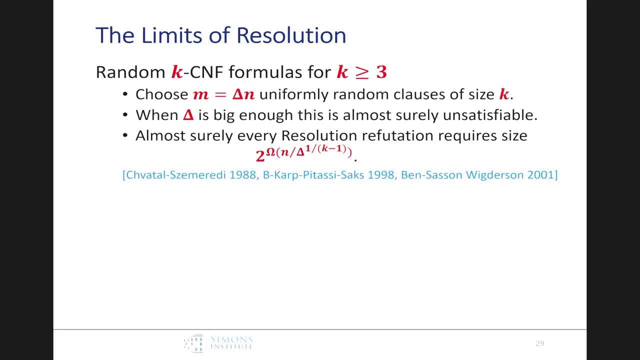 For K bigger than or equal to 3. So that by KCNF that means the clauses are of size K And if we choose some linear number with a sufficiently large constant in the linear number, it's unsatisfiable. almost surely, But almost surely, every resolution refutation requires exponential size. 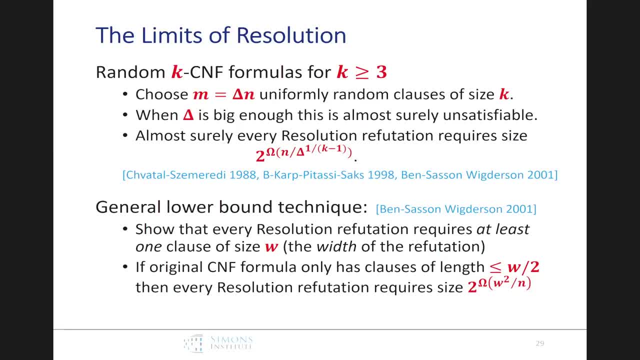 So there are loads of other problems that one can show resolution is bad at. There's a general technique, due to Bensasson and Wigderson, That if you can show that there even has to be one large clause, one clause of big size, 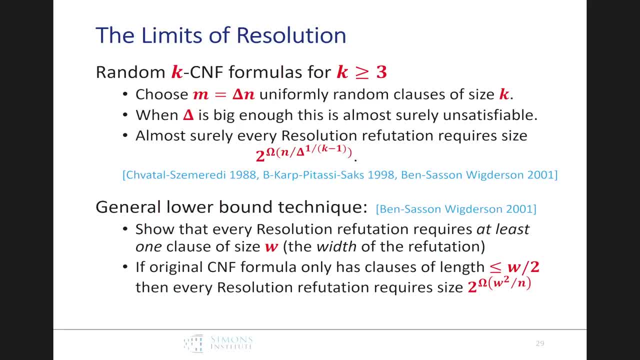 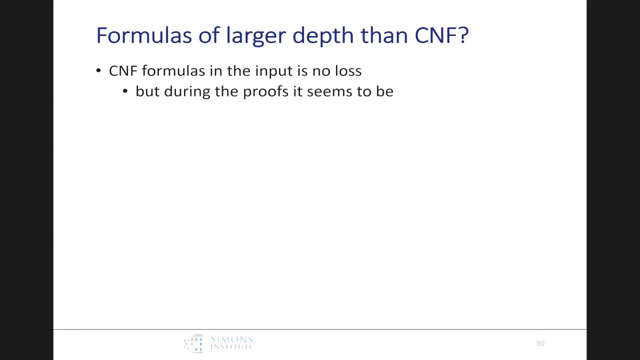 then the whole proof is huge, provided the input doesn't have clauses that are too big. But we'll think resolution and random formulas we'll kind of think of as a little carrying examples, But they're just representative of many other examples that are known to be hard for resolution. 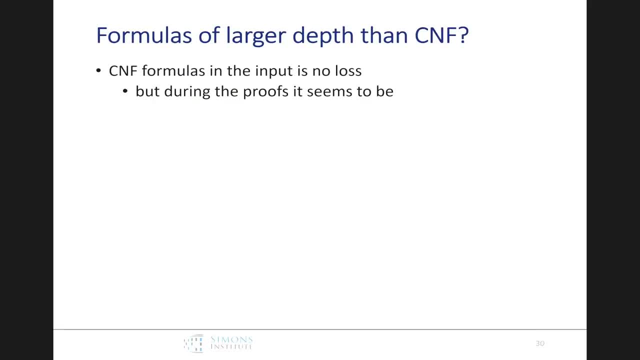 OK. So what about formulas of larger depth than CNF? Well, CNF input was no loss. OK, But it seems potentially that requiring that in the proof is a loss. What happens if we allow a little bit more? So CNFs are big ands of big ors. 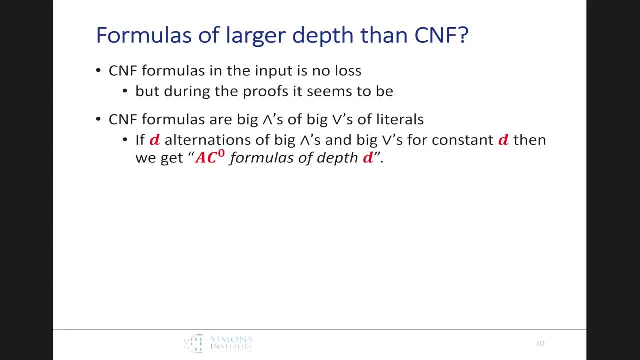 What happens if we have big ands of big ors of big ands of big ors D levels deep? then we get AC0 formulas of depth D And no, they can't do the pigeonhole principle either. It's still exponential for them to prove the pigeonhole principle. 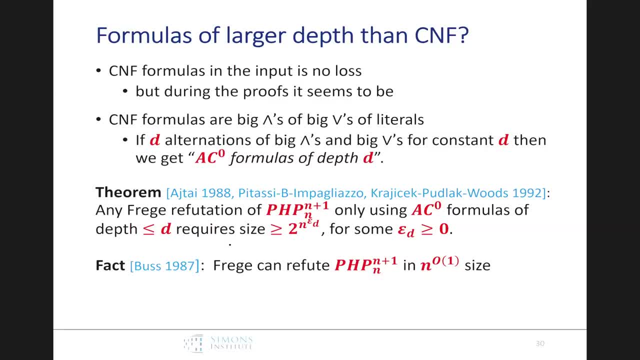 Now it is true. It's true that Frege proofs can actually prove the pigeonhole principle in polynomial size. We'll see in a minute why I'm not going to talk too much about Frege proofs. But one thing that's still open for these bounded depth proofs is whether random formulas 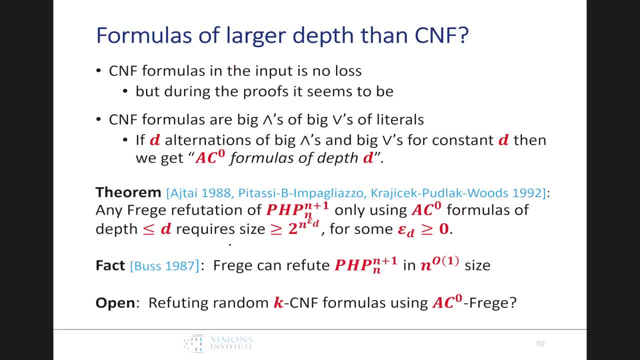 have. even have efficient proofs, It's still open that random formulas, these random KCNF formulas, might be hard. So these are systems that are more specialized in Frege. What happens if we go in the other direction, to get more general than Frege? 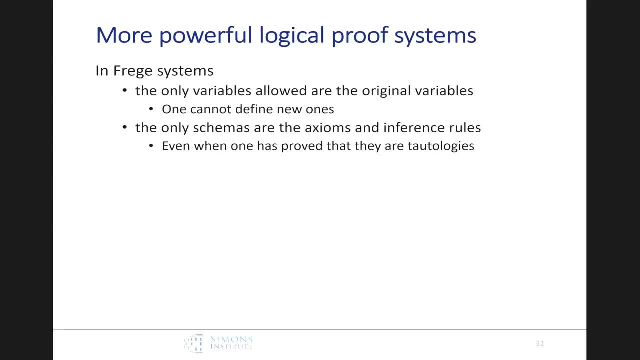 So in Frege systems the only variables that you're allowed to use are the original variables. You can't define new ones, And the only schemas you get to use are the axioms and the inference rules. But suppose you proved an axiom. 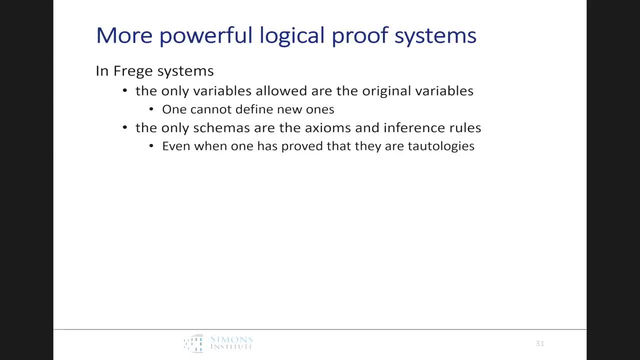 Why not allow yourself to substitute in that axiom right away? Suppose you proved a tautology, Why not allow yourself to substitute into that? You could do that, that too well, if you allow either of do these two things: substitution of arbitrary formulas, or extension where you allow extra variables, even if you've 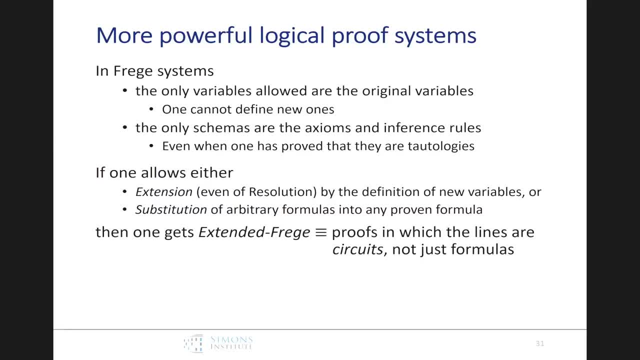 started to adjust with resolution. then it turns out you get a system called extended Frege, and cook and Reckow actually proved that all extended Fraga things are equivalent proofs in which lines are basically Boolean circuits and not just formulas. and in fact this extension of resolution is. 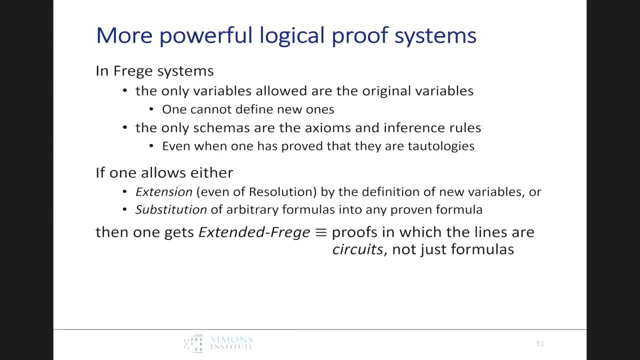 kind of a natural direction that people have tried to do with practical SAT solvers. their limit it's fairly limited in how well it works so far because the trying to figure out how to define new variables is really hard for the search. but we don't have to stop here. we can even define proof systems with 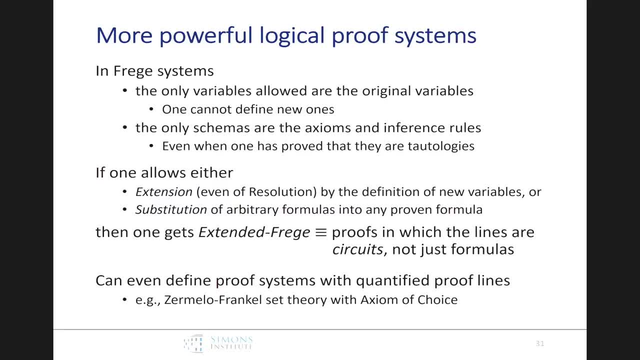 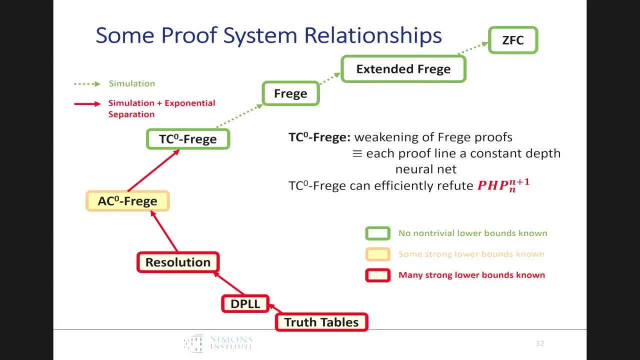 quantified proof lines. hey, why not do Z? there's your mellow Frankel set theory with the axiom of choice. that could be a proof system. so if we take in these directions, here are some proof system relationship we know. so truth tables. DPL l resolution. 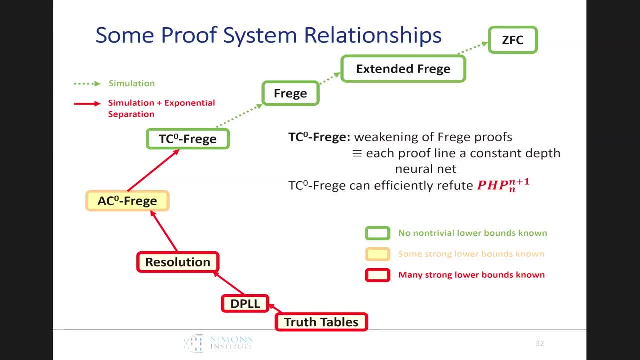 ac0, Fraga and zfc and there's no reason to see say that it stops here. we don't believe that there's actually any stopping. there might be an infinite family of more more powerful proof system. there's one I haven't mentioned here, but this is TC 0 frage. it's a different weakening of a Fraga proof. 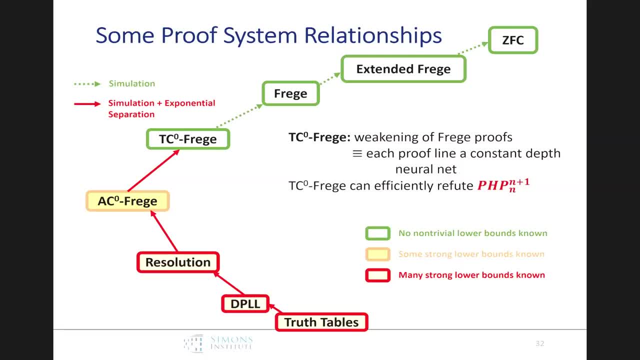 each line here consists of a constant depth neural net. basically, they can count, so they can do pigeonhole principle. and the reason why I didn't say anything more about these is we have no idea about lower bounds for any of these systems up here, so we're going to focus on systems. 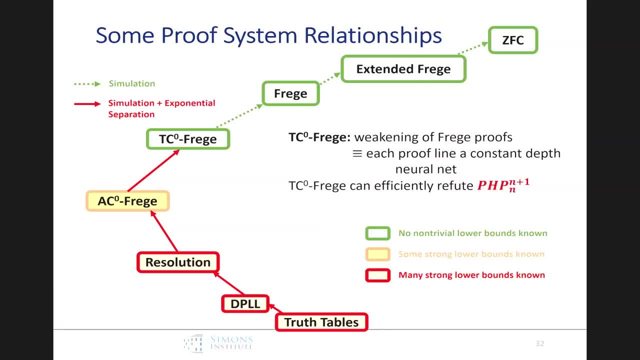 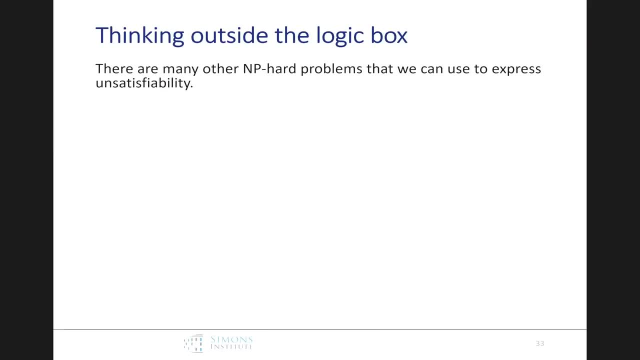 where we can actually do some analysis on them now. well, let's think outside the logic box. there are many other NP hard problems that we can use to express the problem of unsatisfiability. that's one of the nice things about the completeness of SAT or, equivalently, the completeness of unsat. 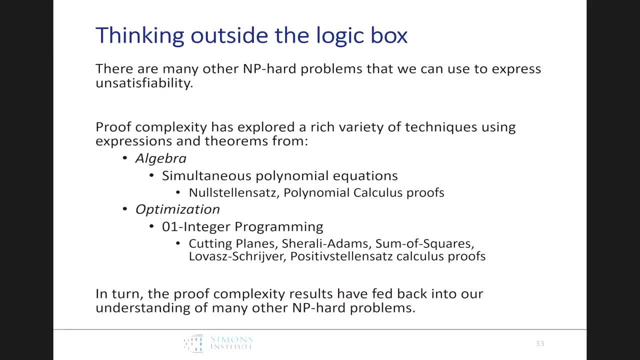 so. so proof complexity. a lot of the work in over the last couple decades has been exploring a rich variety of techniques using expressions and theorems from algebra and from optimization, and we'll go through some of these proof system and one of the nice consequences in turn, the proof. 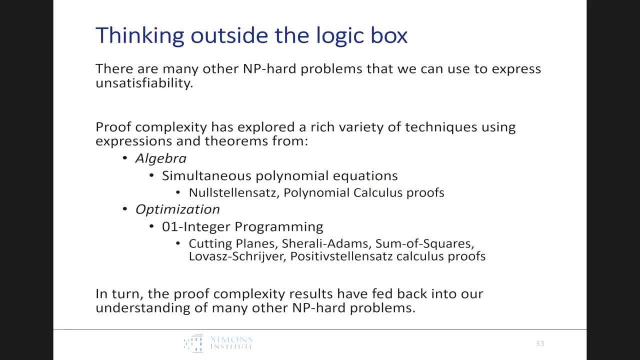 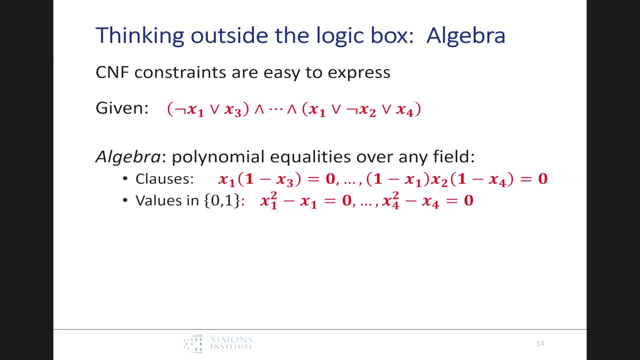 complexity results have actually fed back into our understanding of these other NP hard problems. so let's start with algebra. well, in algebra we can take these clauses, and this is where CNF is especially nice. we start with clauses and we can convert them to polynomials. so this polynomial evaluates to zero if, and only if, X 1 is 0, so not. 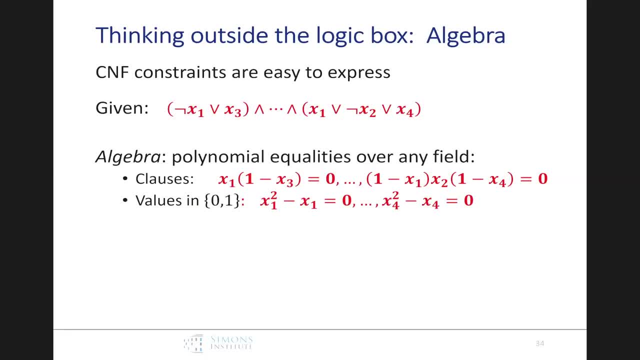 X 1 or X 3 is 1, and we can do similar things for the others, so that exact, and we add the the constraints that every variable is equal to its square, which guarantees that things are either 0 or 1.. it turns out there's actually another translation that might be even nicer, which 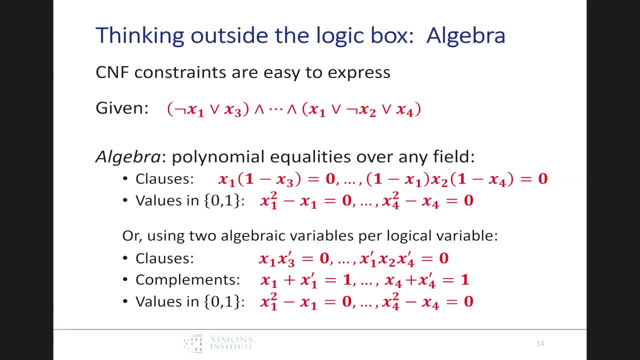 is to put two variables for every original variable, that they're 0 and 1, and one is the opposite of the other. so X prime is like the is kind of the analog of X 1. prime is the analog of, not X 1, and so we can just do a direct. 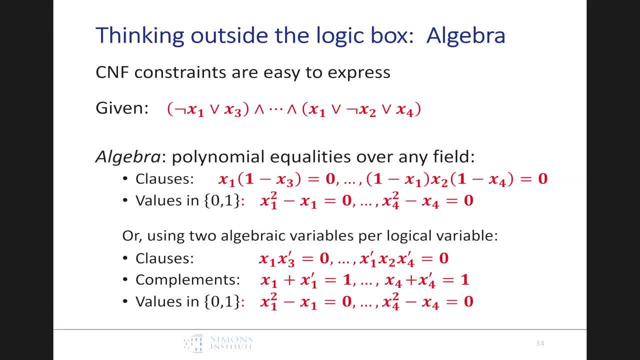 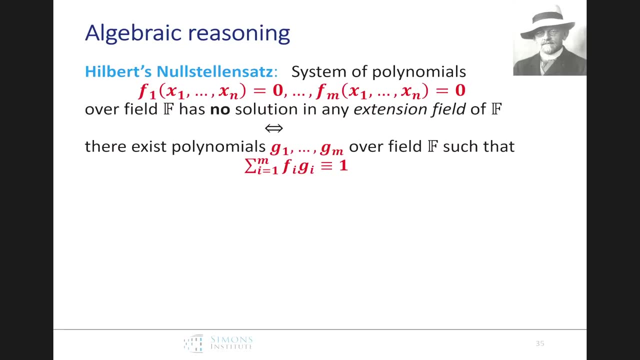 interpolation of the clauses and if we multiply things out. the nice thing here is that we don't get big terms when we multiply them out, so, um, so how do we reason with these algebraic systems? well, here goes our friend, uh, David Hilbert. uh, again, um, in the work before he got into, uh, logic. 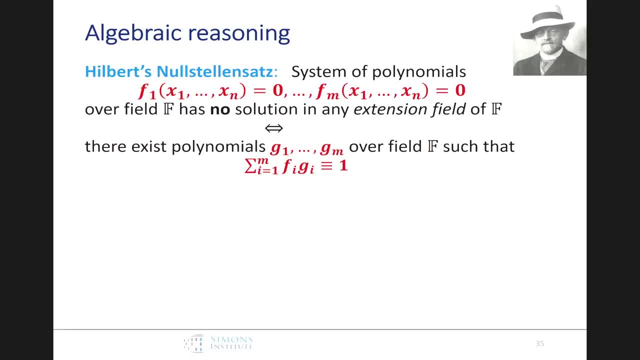 and proof, he proved his famous notion thoughts, of which this is a simplified special case. so we started with a system of polynomials like the system that we generated from the clauses. that system has no solution, so it's unsatisfiable and me in any extension field. 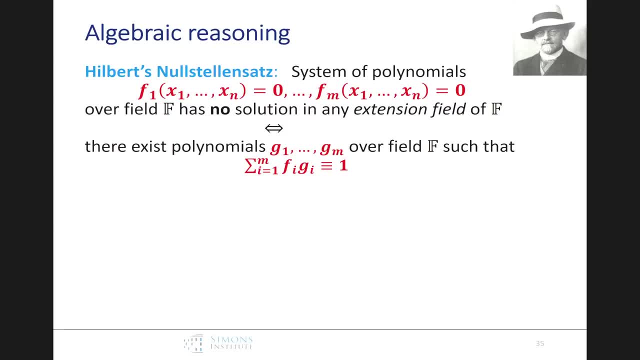 if, and only if, this, if there exists polynomials over the ground field, such when you take that linear combination you get one or one is in the ideal generated by these original polynomials, the abstract way you'd say it. but we actually want to write down and think about what these uh. 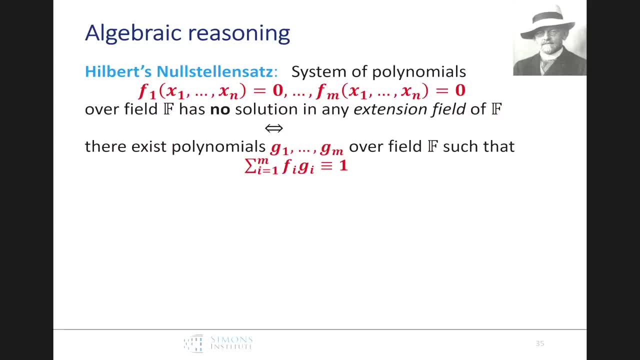 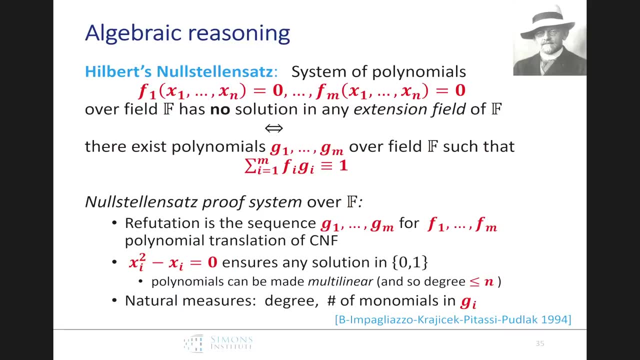 polynomials are, and with this you can get a one system- no, Stalin's proof system- over a field F, and so you get a different one over every field. the refutation is this sequence of polynomials G1, true, GN. why is it a refutation? I should have mentioned this. well, if all of these polynomials are zero, no, 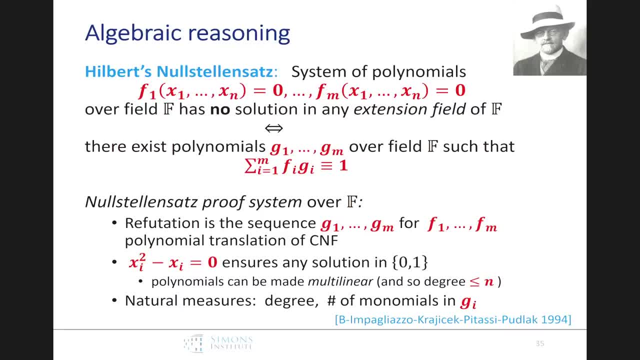 matter what the gi's are, you get a left-hand side of zero and a right-hand side of one um. so the other thing that's that's nice is this: xi squared minus xi is zero. ensures that any solution is zero one, so you don't need to. 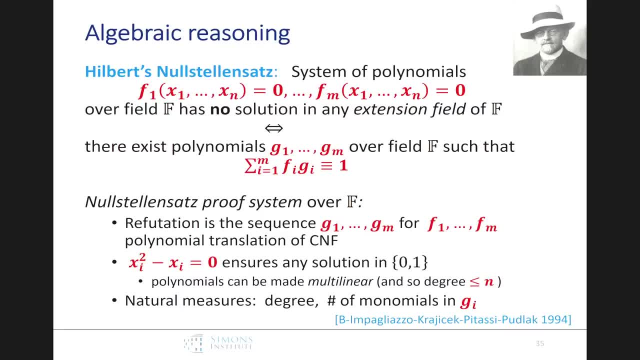 go to any extension field and it also ensures that we don't have to think about degrees in any variable larger than one, so they're multilinear in the total degrees at most end. so this is one way one could take Hilbert system and make a proof system of it. just write down the gi's and check. 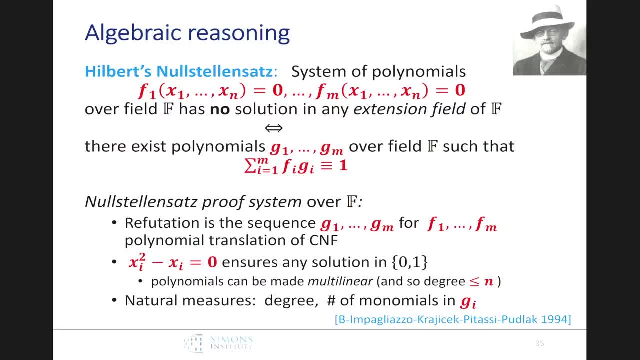 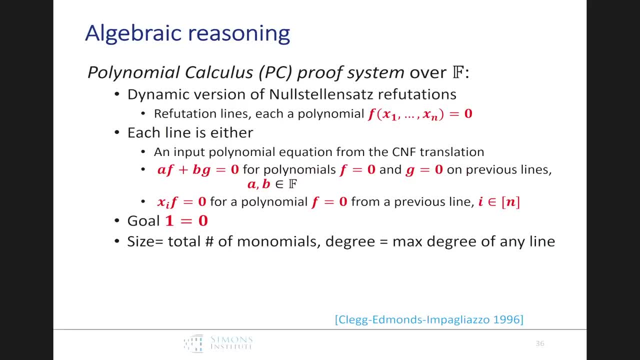 just do the the polynomial, multiply them out and check um. another system that's uh more interesting is what's called polynomial calculus. it's a dynamic version of these notionals reputations. these refutation lines are each a polynomial or a polynomial equation, so it's either an input polynomial. 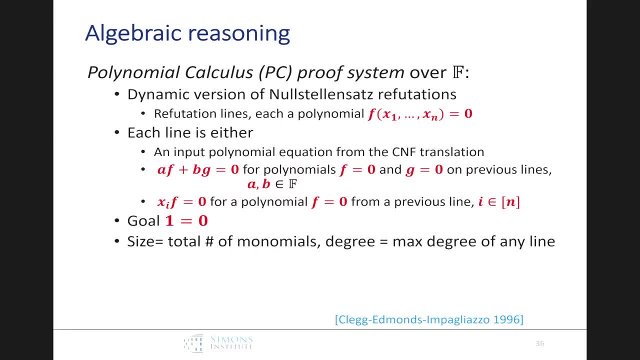 equation. or if you have two previous lines that are both zero, then you should know that their linear combination is zero for any two elements of the field. or you can multiply by um, by a variable um, given a polynomial, and the goal again is to derive that the polynomial one or that one is 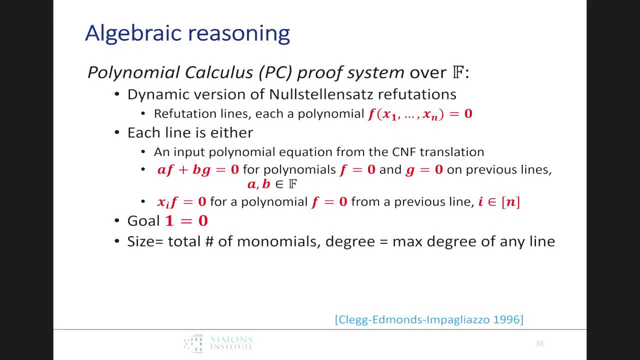 equal to zero and the size here. well, you got to write down these polynomials somehow, so let's write down. oh sorry, uh, yeah, we've got to write them down, these polynomials. so the total number of monomials, or the degree um, which is the 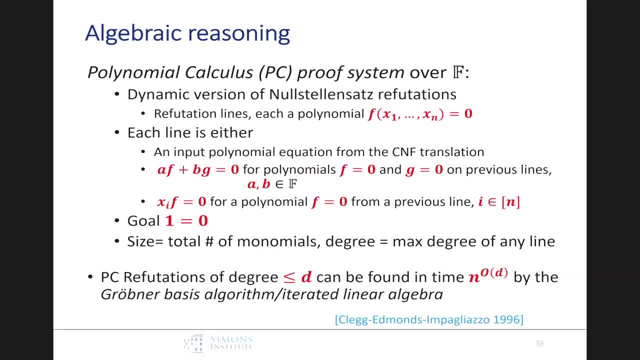 maximum degree of any line. so, and Clegg, Edmonds and paliazzo proved that there's actually a relationship between these two. if your refutation is a degree at most d, that actually can be found in this time, and of course the number of monomials has to be at most end to the D. uh, just by simple. 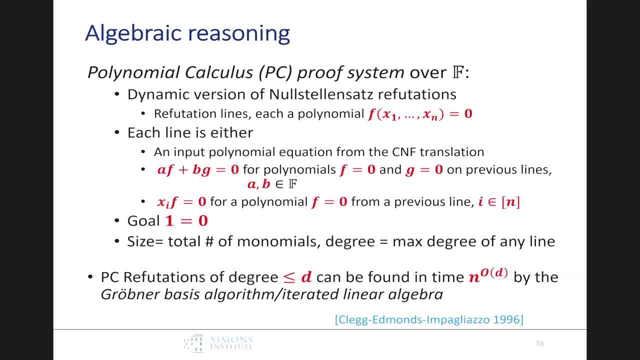 counting. uh, and the algorithms that do this are grubner basis algorithm, which you can think of as iterated linear algebra. but the grubner basis algorithm is a very useful algorithm of people's apply in practice and it turns out polynomial calculus exactly captures the capabilities of 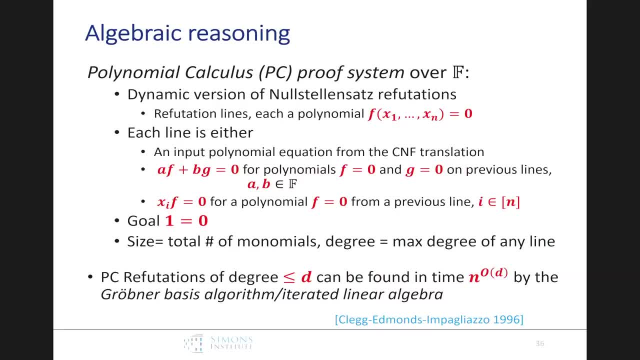 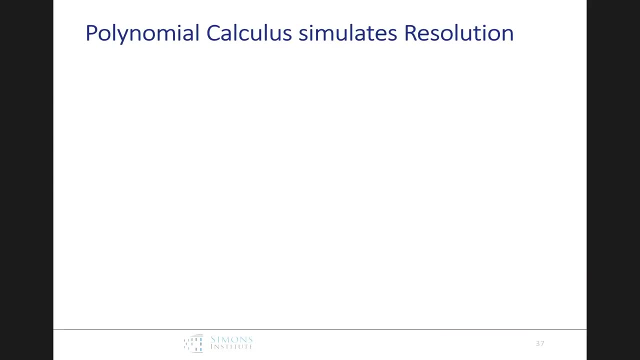 this Grubner basis algorithm. so so this is another proof system where the proof system really nicely matches what's going on in practice. well, for both of these systems there are some. well, first of all, polynomial calculus nicely simulates resolution. I thought I'd include one simulation slide. I'll do it in the two variable form, so if we've got some, a couple. 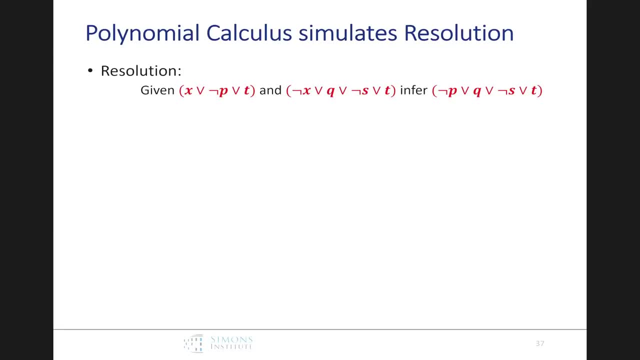 of clauses, we've got X and not X, and this is the thing they're supposed to infer. here's a typical proof. so we do the translations with the two variables. we just multiply by the constant terms. I've done a few steps. we add them up, we use the given, we add them up and we get the final line. 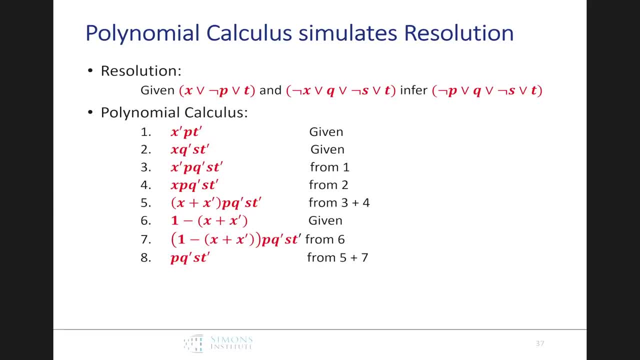 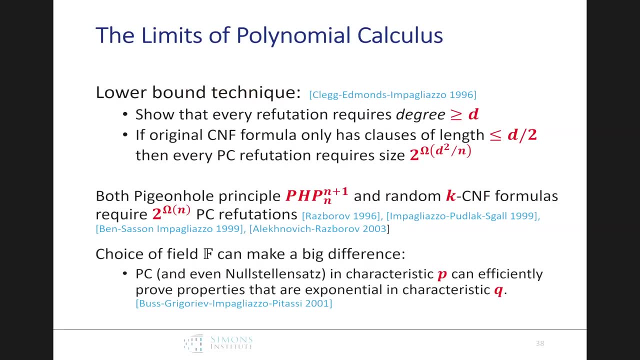 so fairly straightforward, and this is very typical of the kinds of simulations that we do in practice. so I'll do it in the two variable form. so if we've got some simulations, one can get now. there are limits to polynomial calculus. in fact, Clegg, Edmondson and 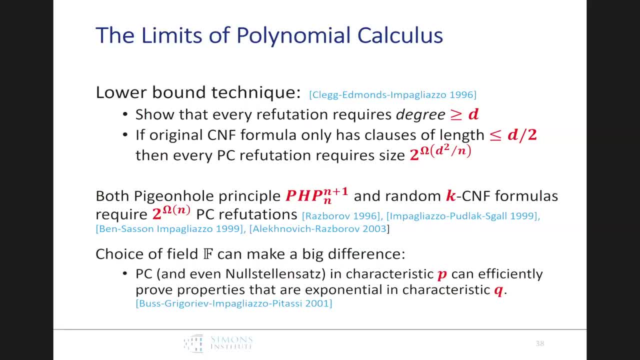 Pagliazzo showed something just like we been. Sasson and Wigderson had a result for width of CNF formulas implying that if you've got one clause that's big, then the whole proof must be big. in this case it's: if you've got one big degree term, then the whole proof is big and in 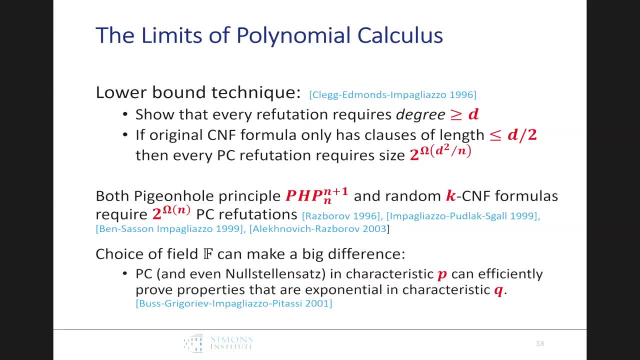 fact Clegg, Edmondson and Pagliazzo did this proof first and Ben Sasson and Wigderson adapted it to the case of resolution. unfortunately, both the pigeonhole principle and random KCNF formulas require exponential size. refutations didn't help too much, but here is an interesting thing. that's a bit. 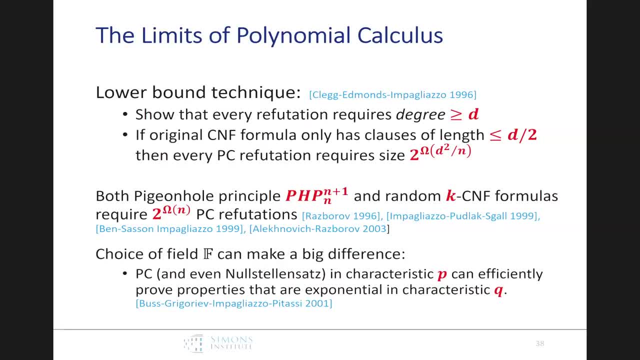 different, but from before the choice of field F can actually make a big difference. so if you're in characteristic P, you can efficiently prove that you've got one clause that's big, and if you've got two properties that are exponential in some other characteristic Q. so we get a complex system of 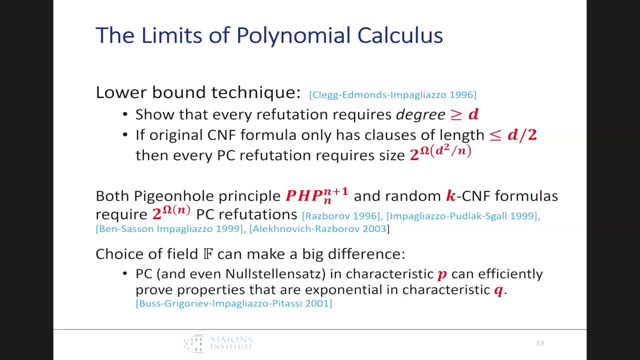 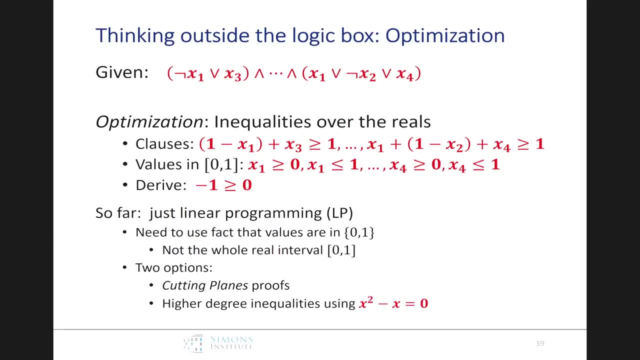 relationships among different proof systems for different fields, though for most of the rest of this I'm going to focus on the case of the field being the rationals of the reals. let's go to another direction of thinking outside the logic box. so, optimization, so we've got our. 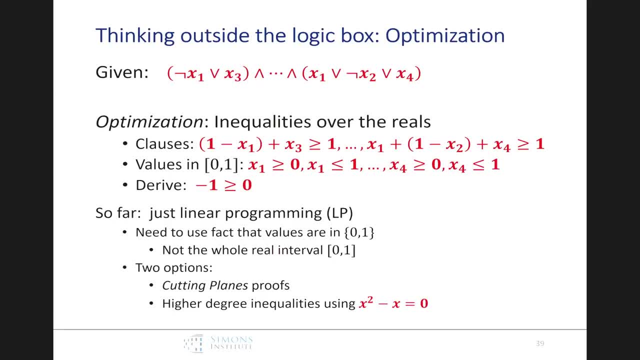 same formula here. we replace each literal by an expression. negation is one, the positive form is just the original variable, negation is one minus it, and for every clause we just say the sum has to be at least one. we've got to add, of course, the fact that these variables are between: 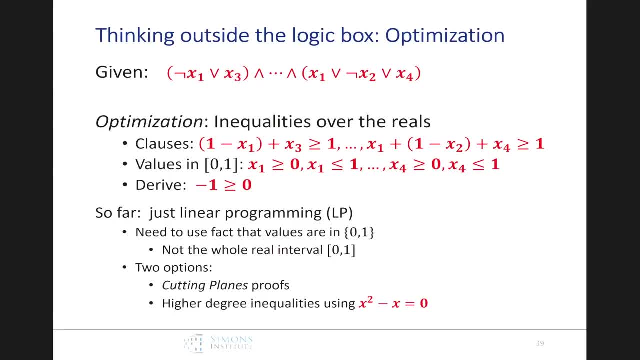 zero and one, and our goal is to derive that negative one is bigger than equal to zero as formalized here. this isn't enough. this uh is just linear programming and it doesn't prove properties that are true just over zero one. it it's the properties over the whole interval of all values between zero. 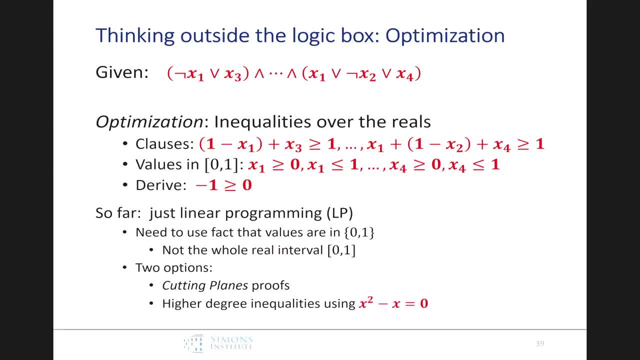 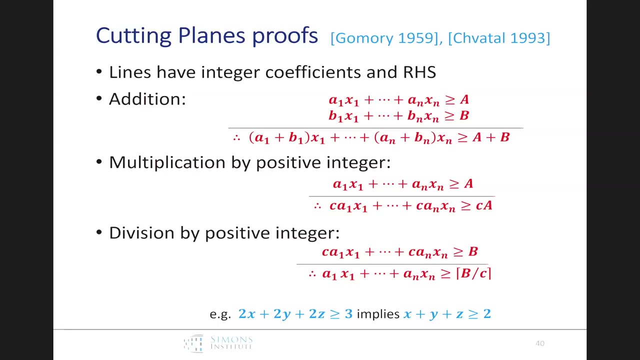 and one. so the input formulation doesn't give us all the information we need. so there are two options and two directions of proof that people have used. one is cutting planes proofs and the other is higher degree inequalities, using this xi squared minus uh, x squared minus x uh system. okay, so, um, what are cutting planes proofs? um, so these go back a ways. 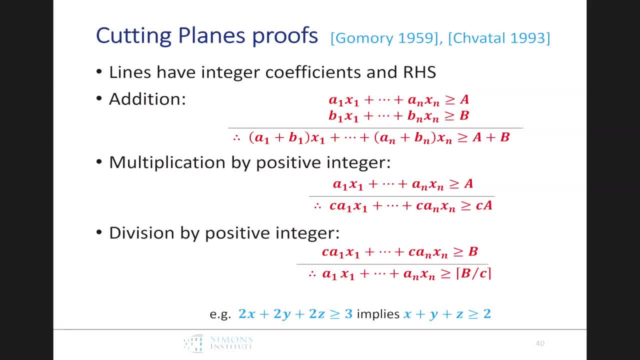 to work of gomery in 59 and kvartal actually formalized it as a proof- system for integer programming. so lines have integer coefficients and integer right hand sides and we've got rules of addition, the usual rules that we have, uh, for addition of inequalities and multiplication by 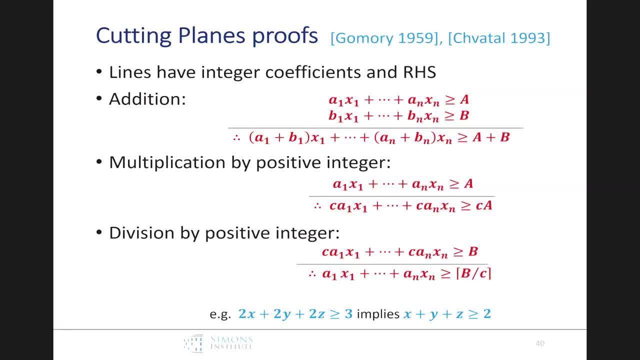 positive integers, so it doesn't flip the sign. these things don't actually take us beyond linear programming. the key thing we need is this division rule: we get to divide by a positive integer, so if we've got a common factor c, we can divide both sides by c and then round up. and this is 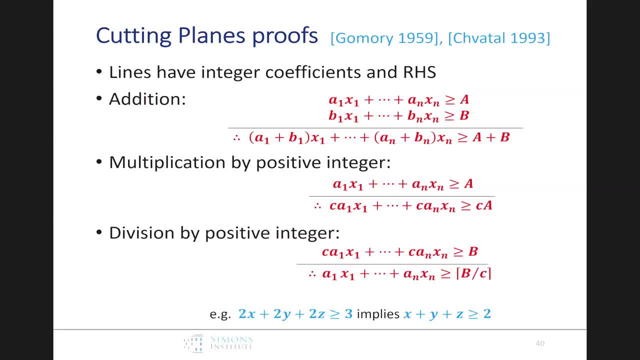 only true, because things are interesting is if we can multiply both sides by c and then round up, then we would get x, q, the final definition of the equation, and then we would get the relation of equaliate to absolute algorithm of the equation. so now let's look at the solution on the following slide. 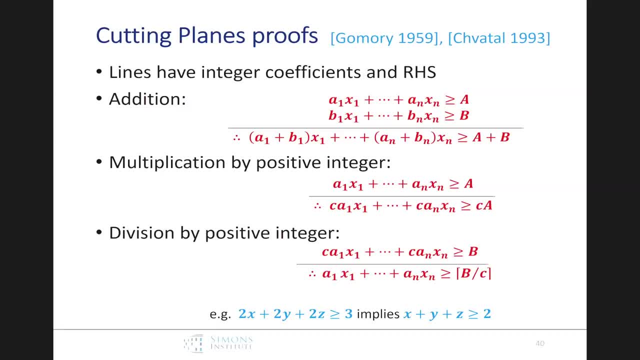 there is aciót of e. i is only the three-dimensional solution of the equation. so we're only the three-dimensional solution of the equation, but now there are three-dimensional solutions of the equation like a bit like cutting planes, so far as uh, jacob nordstrom and others have shown. 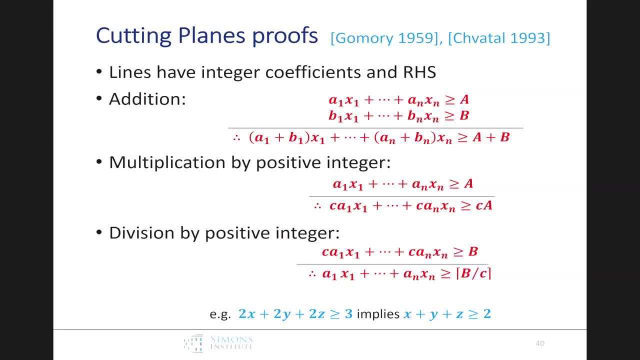 their limitations. they haven't yet been able to get to the the power of full cutting plane system. i'm not going to talk about the limits of the system specifically, i'm just going to go on to the other method. oh, why is it called cutting planes first? so it's called cutting plane so. 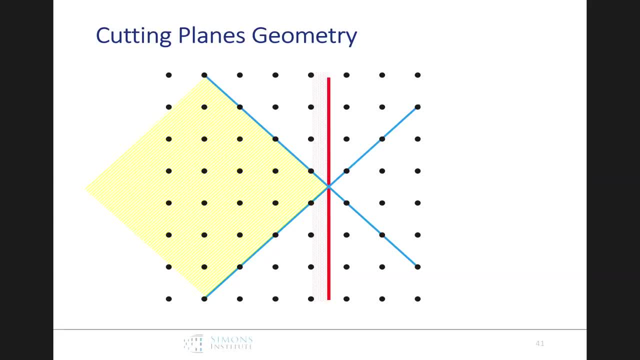 here's why. basically, when you do that random linear combination, let's say, if we take these two inequalities and we just add them, we get this inequality. so here's the region that these inequalities give you- we get a new one that says everything is to the left of that line. 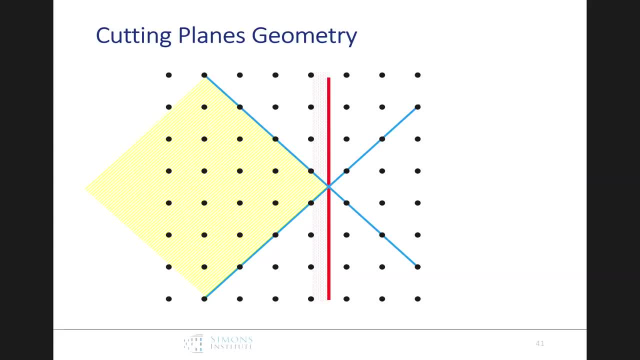 um, and what cutting planes allows you to do? the rounding essentially lets us shift that line to the first integer points that are going to be involved there, and we get to cut into the side of the polytope. so that's why it's cutting point anyway. so we're going to go on now. 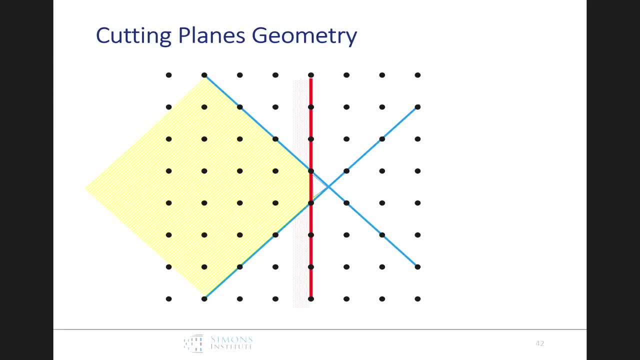 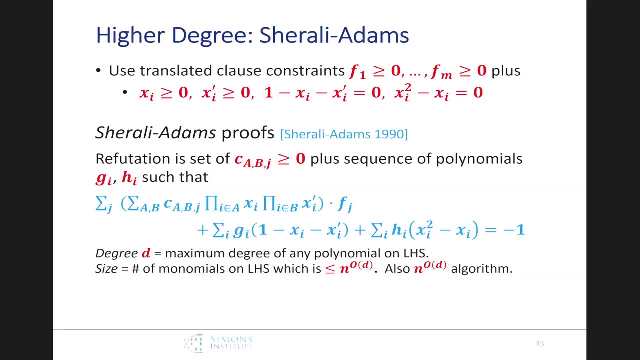 to high um and we're going to go on to the next one, which is the, the other method for ensuring zero one and one of them, which i know a number of you will have seen, the shirali adams proof system, but probably not too many in the format i'm going to strive here. 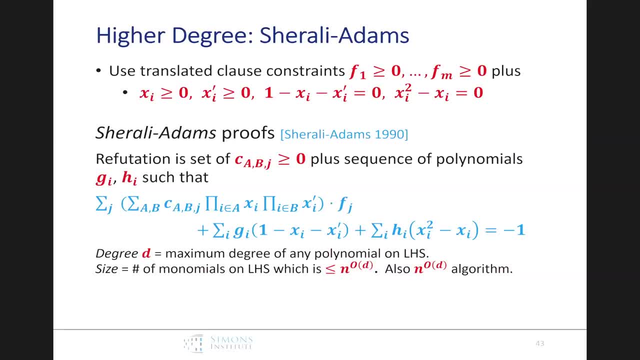 it's completely equivalent. so the general idea here we're going to use that two variable translation. so i'm going to stick that in just to make it more convenient to write down and fit on our algorithm. a z of three and i'm going to go with. so this represents a. 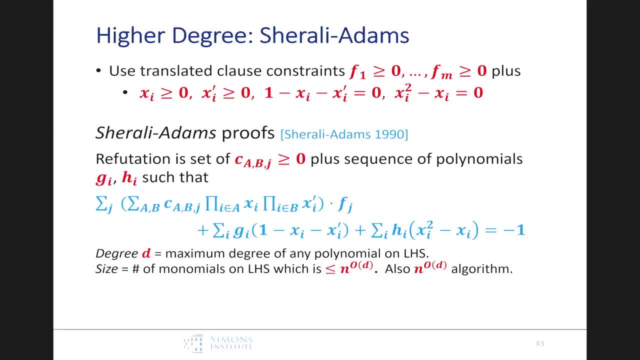 These things are non-negative. Both of these are bigger than, or equal to, 0.. And this is bigger than, or equal to, 0. So we've got these conditions. That tells us the left-hand side. well, this part is 0.. 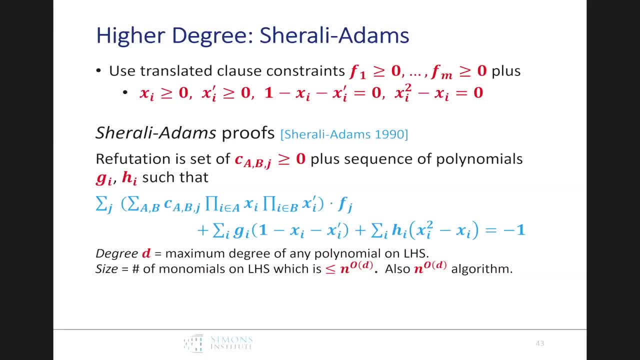 And this part is bigger than or equal to 0. So we're saying negative 1,, which is supposed to be equal to all of these things, is bigger than or equal to 0, an obvious contradiction. And again we can talk about the degree. 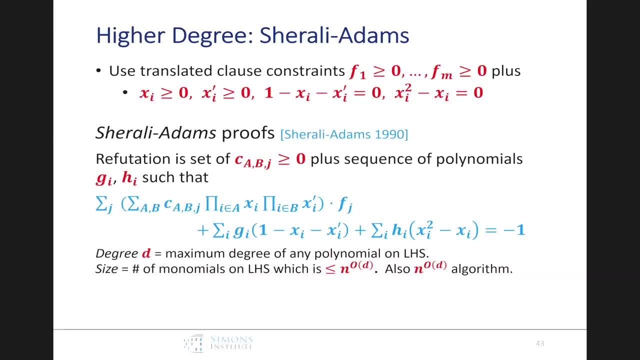 how big a degree did you need to write it down? and how many monomials? And again, there's an n to the order d algorithm to actually find these Schiralli-Adams proofs. So that's one method of doing it. 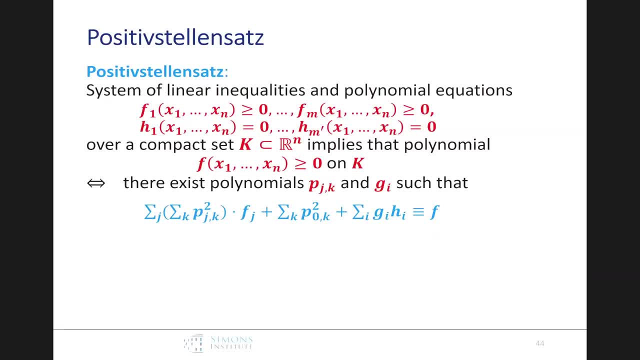 Another method of doing it is to use the generalization or ageneralization of Hilbert-Schnoll-Stellensatz to the positive Stellensatz. So here I'm going to state a very restricted form. We've started with linear inequalities. 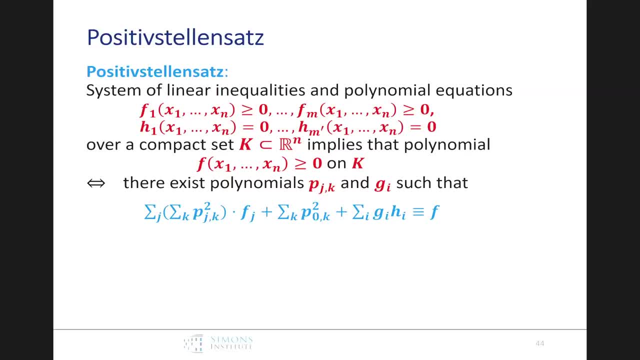 and polynomial equations. So suppose we've got- We can think of these as our original clauses and these are the constraints, And suppose those are satisfied over some compact set. Then that implies that some other polynomial is bigger than or equal to 0. 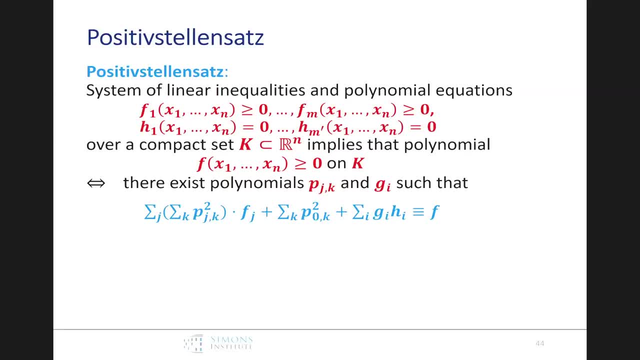 And we could choose that polynomial to be the constant function minus 1, if we were going to refute things, if and only there exists some polynomials p, And we're going to multiply each of our original non-negative transformations And we're going to do the same translation of our clauses. 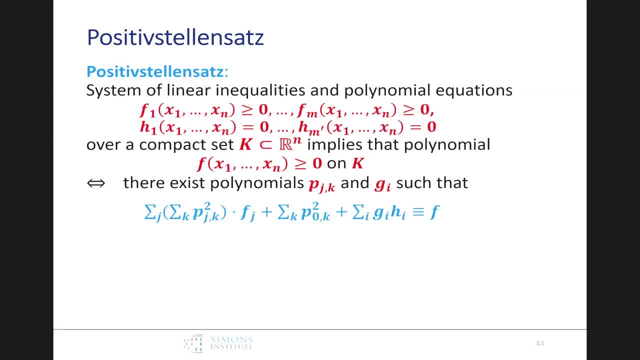 by a sum of squares of polynomials, add another sum of squares, and then we get to do the same sorts of things that we're doing with Null-Stellensatz, And this theorem generalizes the Null-Stellensatz, but only over the reals. 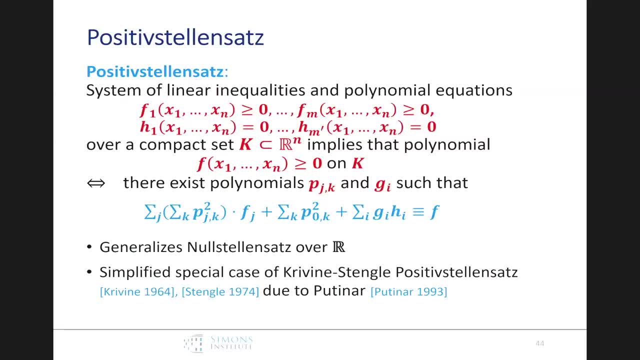 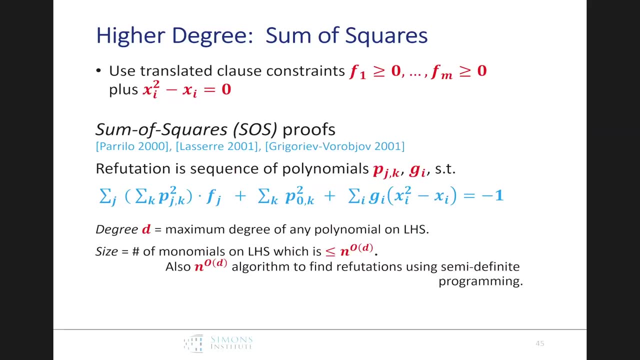 And for those of you who know, here are some references. This is a particularly simple form of positive Stellensatz. There are a bunch of Varied versions, But this gives a proof system and we don't need variables and negation, where we just take that left-hand side. 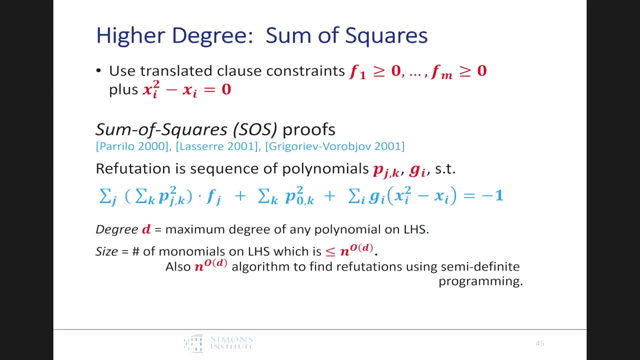 and set it equal to minus 1.. And this is the sum of squares. proof system, which more or less was under equivalent names, was independently invented around 2000.. The names were used were positive Stellensatz and other people called it Lasserre. 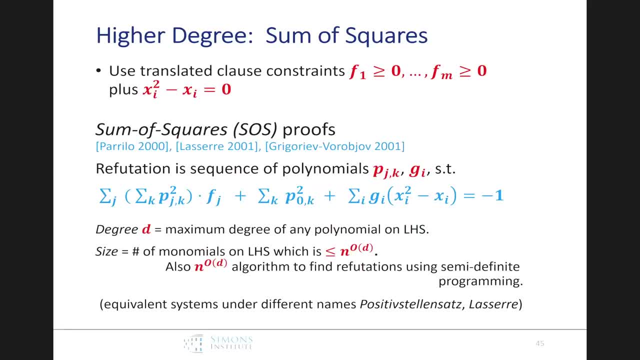 I don't think he was there. He was doing that. So anyway, sum of squares, proofs on many in the room know have been of huge interest in theoretical computer science in the last, let's say, decade or so and there have been big advances. 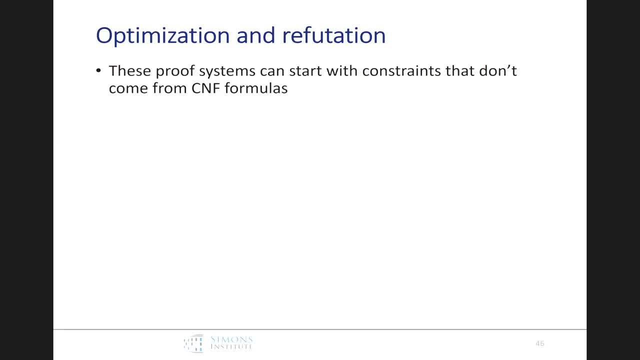 in our understanding of sum of squared proofs, And one of the things that's been important is the connection between optimization and refutation. So these proof systems can actually start with constraints that don't come from CNF formulas, so you can do things directly. 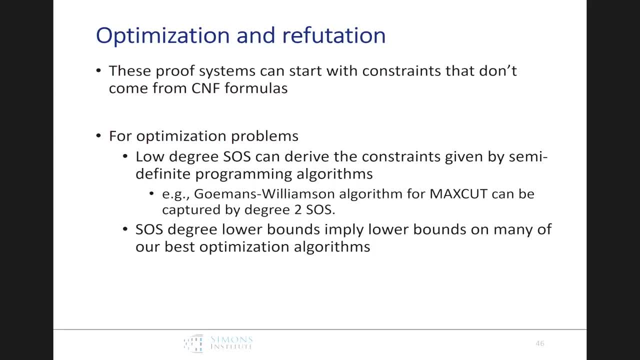 For optimization, low degree sum of squares can derive all the constraints given by semi-definite programming algorithms. For example, the Goemans-Williamson algorithm for max cut can be captured by degree 2 sum of squares. On the other hand, if we're going to do this, we're going to need: 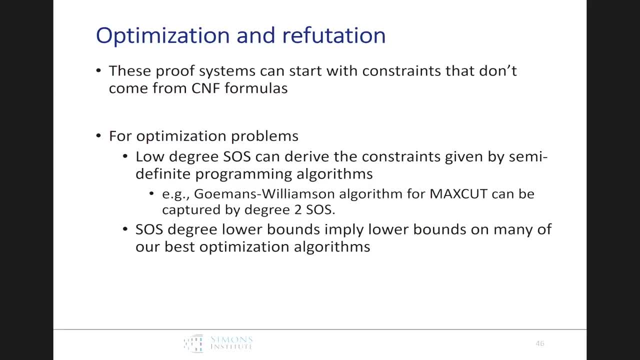 to have a degree lower bounds for sum of squares proofs. That implies lower bounds on many of our best optimization algorithms. So I'm going to go through one example of a class of optimization algorithms that there's been a lot of recent work using proof complexity to understand. 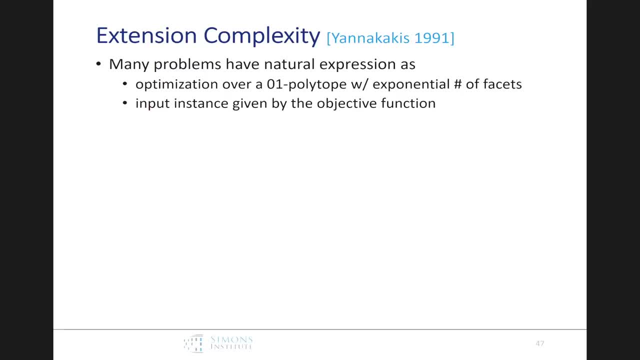 and this is extension, complexity, which was defined by Yannakakis, And the point there is, many problems have natural expressions as optimization. So I'm going to go through one example of a class of optimization over some 0-1 polytope. 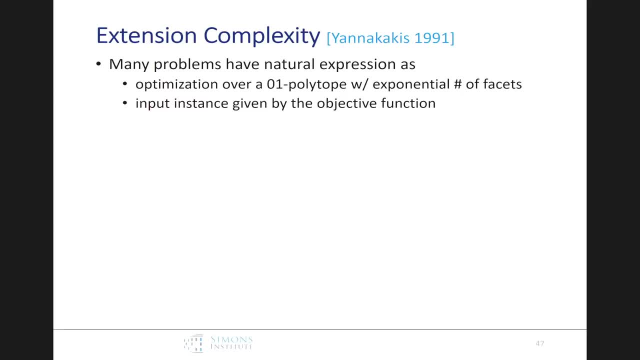 but with an exponential number of facets And the input instance is given by the objective function And I'm not going to go through a list of example problems. but the general idea of the extension approach is suppose you have some polytope, that's given. 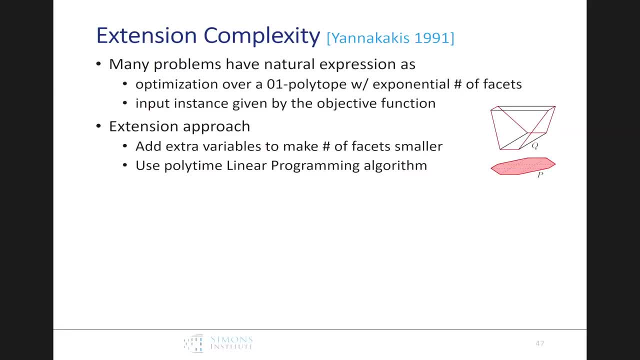 by some very large number of facets. You might be able to add extra variables, go to a higher dimension and end up with fewer facets, because each facet corresponds to a constraint. so it's a lot to write down And then we know. so this one particular has 6 versus 8,. 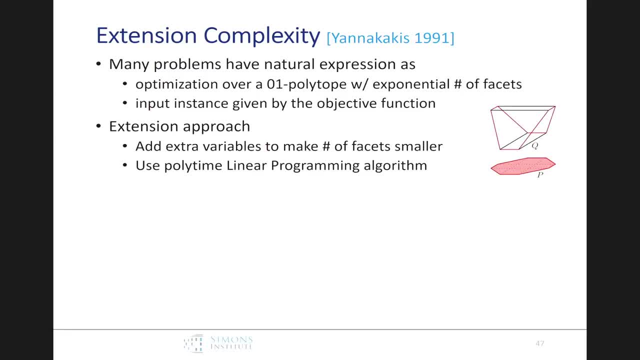 so it tells you you can get smaller. but there are cases where you get exponential speed up And then you could use linear programming up on this upper polytope Q and then just project the answer down to P And relatively so the LP extension complexity is: 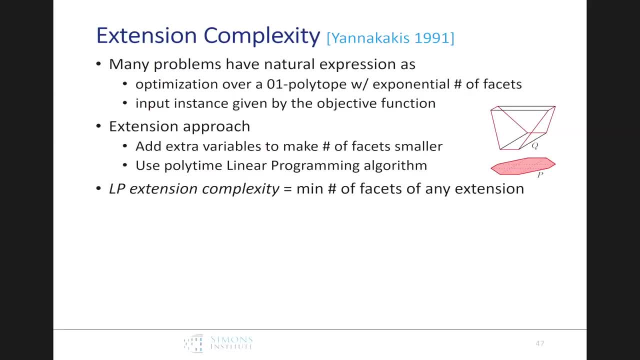 the minimum number of facets of any extension. And Kothari, Manka and Raghavendra, improving on some work of Chen-Li Raghavendra's story, proved that the LP extension complexity of approximating any in a class of problems called constraint satisfaction problems. 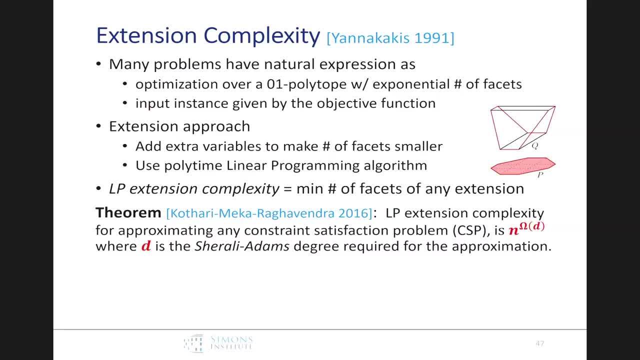 is at least N to the omega D, where D is the Shirali-Adams degree required for the approximation. And as a consequence, for example, they proved that the LP extension complexity of any extension, for example the LP extension complexity for max cut, is only a half plus epsilon. 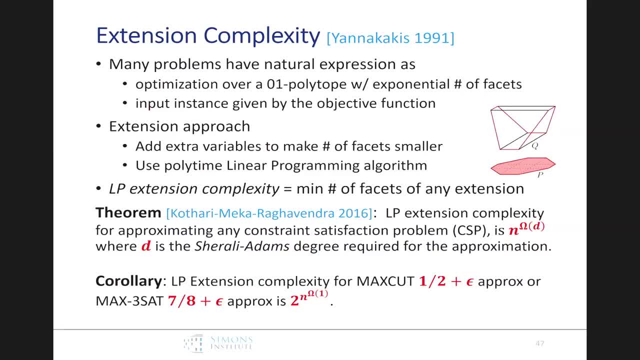 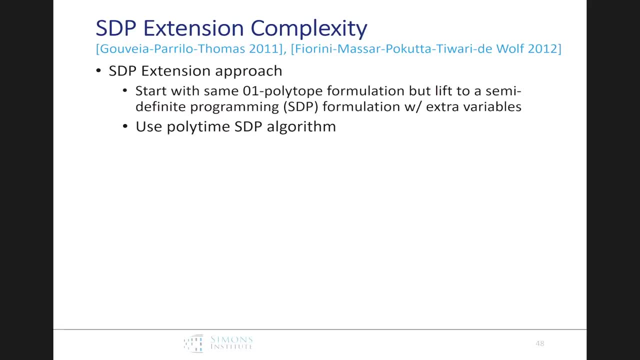 where approximating max three sat is seven-eighths plus epsilon. You can do better, and we know we can do better than this with semi-definite programming. So what about semi-definite programming? There's a version of this that was defined in these two papers. 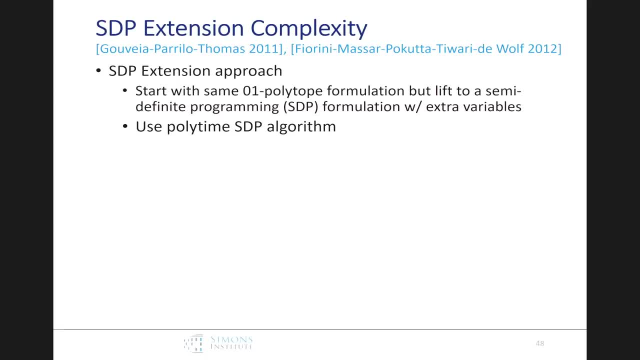 and the basic approach is essentially the same. Start with the same original formulation, but lift to a semi-definite program rather than a linear program with extra variables, and use the fact that we have poly-time semi-definite programming algorithm and the SDP extension. complexity is the minimum number. 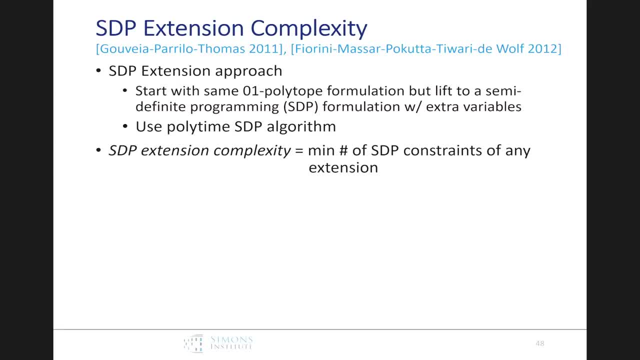 of SDP constraints of any extension. Well, three years ago Li Raghavendra and Storer proved that for any couple of results, first for any CSP, the SDP extension complexity is if, and only if, the degree of doing that, of solving that SDP. 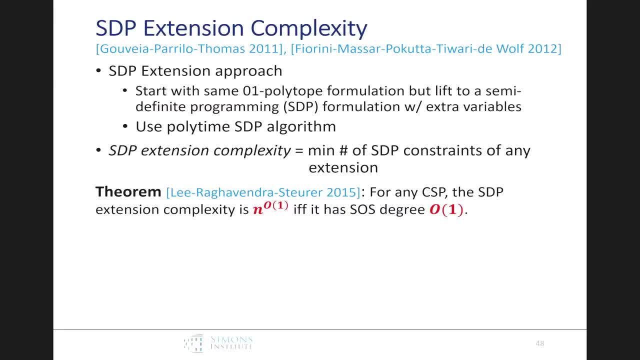 or approximating is also constant. Their theorem actually proved a little bit more, but I'm stating weaker results for all of these than are in the original papers. and the other thing they showed is that the SDP extension complexity of the famous traveling salesman problem, or clique, is two. 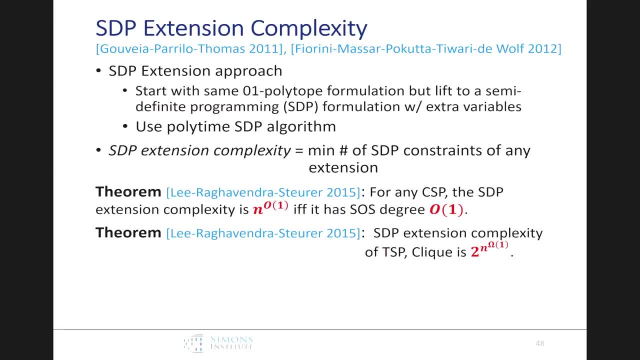 to the end of the epsilon. for some epsilon and, very interestingly, their methods, their proof relies on a result of Grigoriev, on something that seems completely unrelated but is related to sum of squares, which says: if we have an inequality like this, 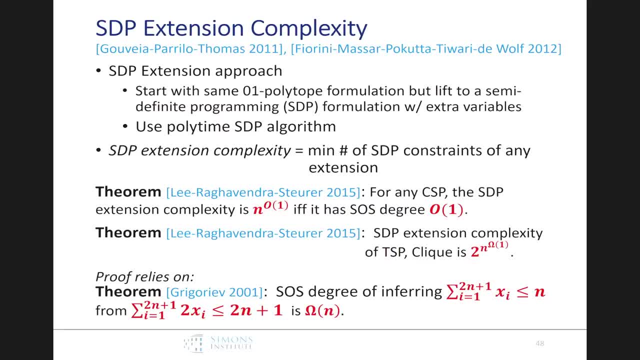 and notice we've got this common factor two on the left-hand side and we want to divide by a common factor two. here it's rounding down. because it's less than or equal to, then you get at most n, and Grigoriev showed that the degree had to be linear. 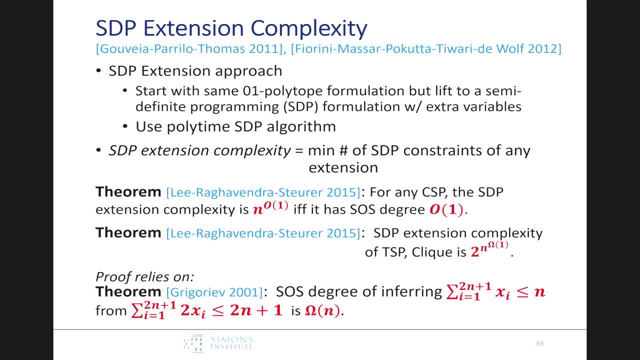 and that's the key textbook. It's the technical result that's behind these stronger results of Lee, Raghavendra and Storrow. So these systems aren't the only algebraic systems we could come up with. they're static systems like Nolstallensatz. 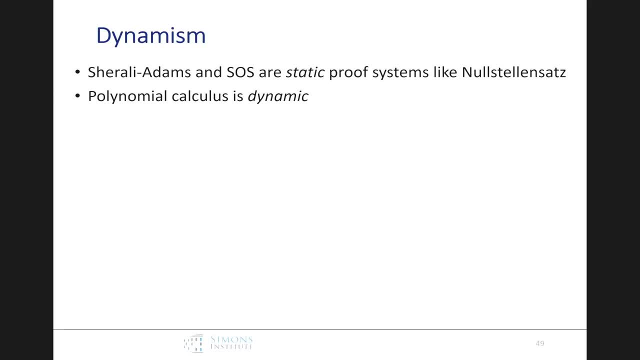 Polynomial calculus was dynamic. Well, very interesting result from last year, in fact, that even though sum of squares is static and polynomial calculus is dynamic, sum of squares can efficiently- you know, efficiently- simulated over the reals. So that's a quite surprising result to me. 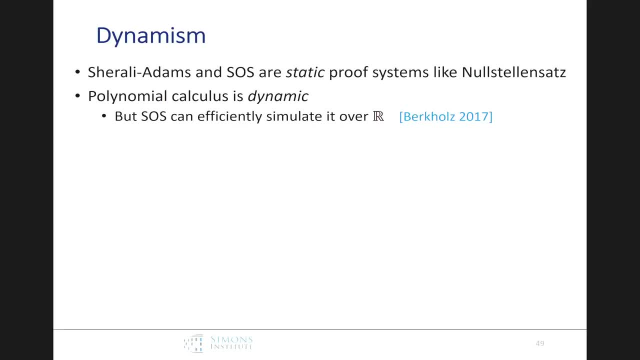 a pretty interesting result. So it says: well, okay, static polynomial calculus is pretty strong, but hey, why not make it dynamic? So we can have dynamic systems for inequality. say, given two non-negative quantities, we can infer: 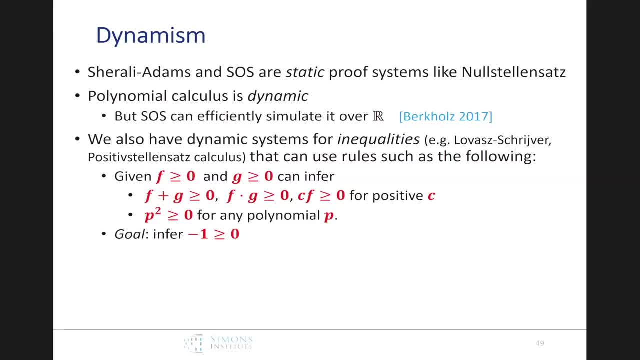 that their sum is non-negative or their product is non-negative. and we could add, you know the square of any polynomial and again the goal would be to infer minus one is bigger than or equal to zero. We actually know very little in terms of lower bounds. 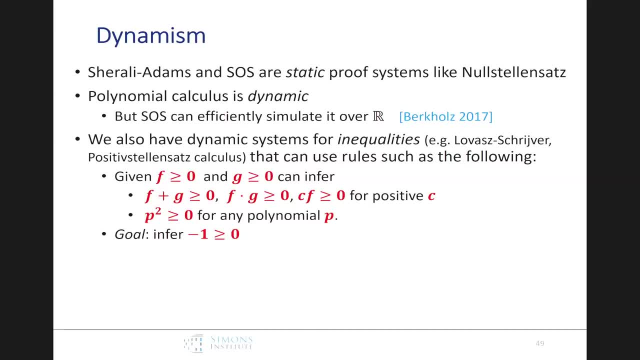 for this system, this class of systems in terms of proof size. we know somewhat more restricted things for special properties and, as far as I know, the best result we know is something like the following: which says that if we restrict this dynamic system to just like that, DPLL to one, 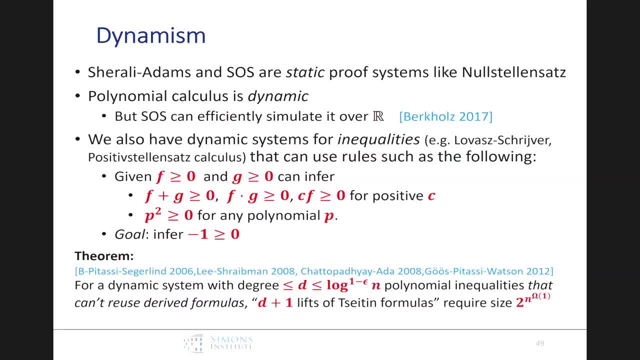 that can't reuse derived formulas, then a certain class of formulas do require exponential size if the degree isn't very big, if it's bounded below log n. So that's it for the general proof systems. Here is kind of a graph of many, I think. 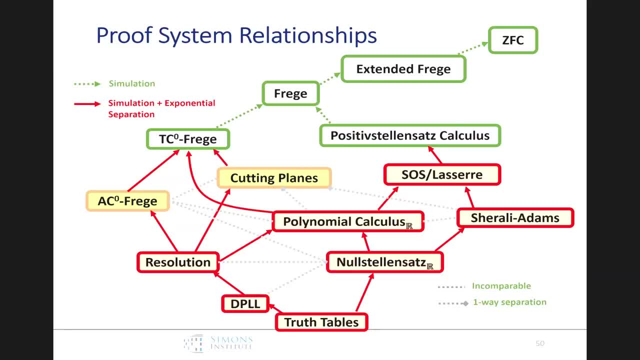 of the known relationships amongst these proof systems. Here, this sum of squares is above all of these and we actually know a fair number of lower bounds for it. We have these other relations. This is one of those dynamic systems and they could all be simulated by Frege. 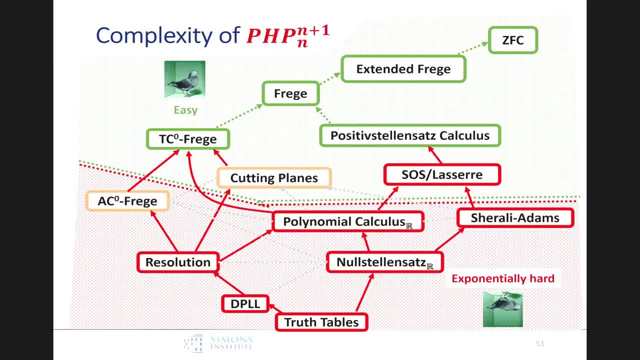 And what about our friend's pigeonhole? Well, we actually precisely know the boundary between the pigeons. actually, maybe the pigeons should be happy down here, Because they can't tell that there's the systems can't tell. But anyway, it's exponentially hard in this lower part. 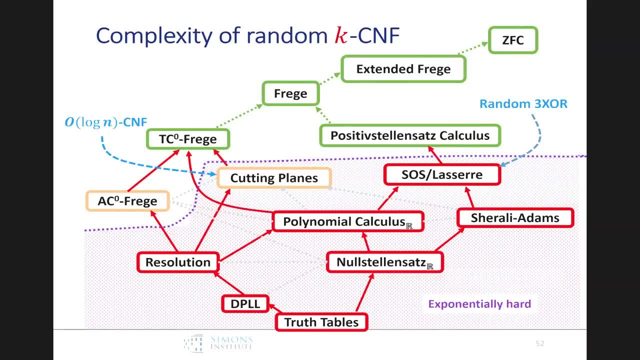 and very easy up there For random formulas. we know a little bit less for it turns out this: random formulas for the sum of squares or Lasserre system actually even holds is even hard if we have random 3XORs and that turns out again. 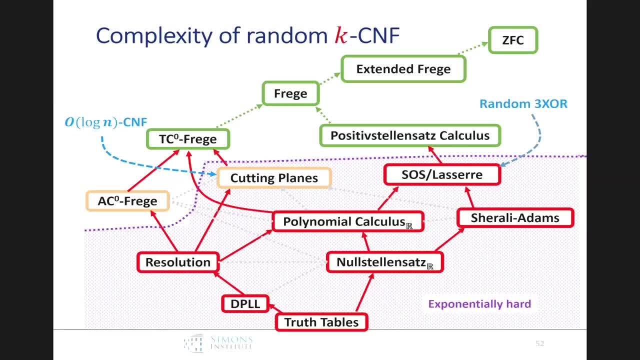 to have surprising consequences. you can prove that lots of NP-hard problems require large sum of squares. proofs based on just the, on reductions from this random 3XOR problem And cutting planes. it's a little bit, it's not quite as. 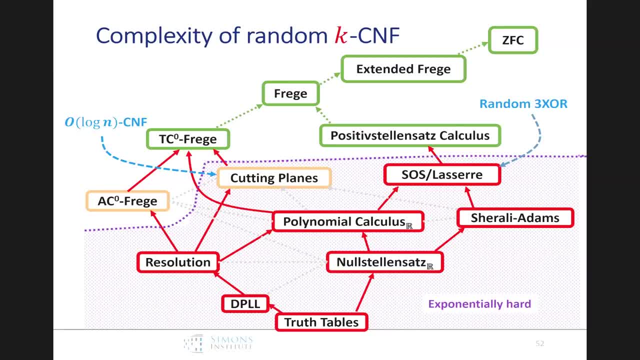 you know we can't prove it for three. What's interesting about random formulas? they're not known to be easy for any proof system, So maybe I'll do a little bit more of that. Maybe they're hard for TC0, Frega, ZFC, we don't know. 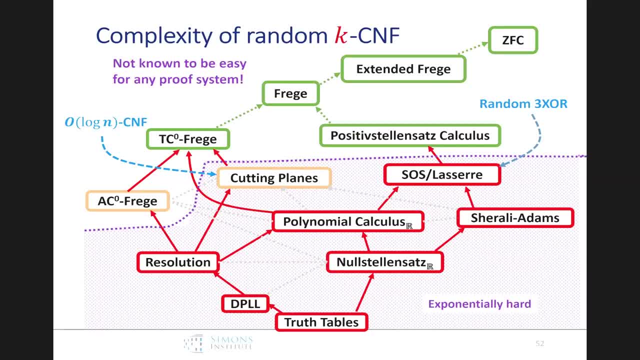 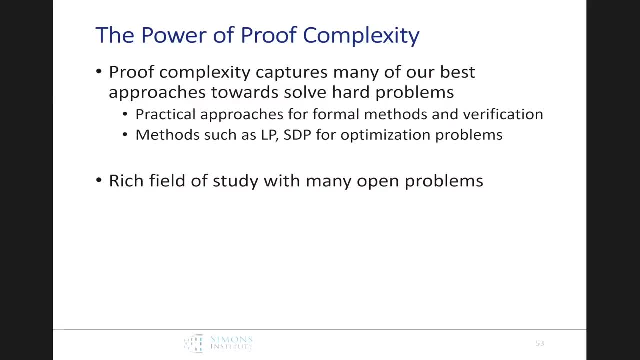 So so that's one challenge. So, in general, proof complexity captures many of our best approaches towards solving hard problems. It covers practical approaches for formal methods and verifications, methods such as linear programming, semi-definite programming, for optimization and, you know, come join the working on this field of study. 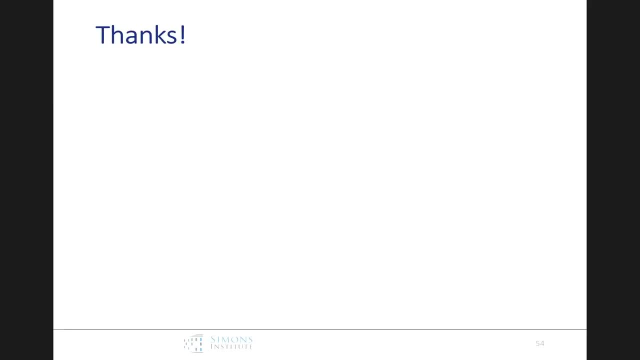 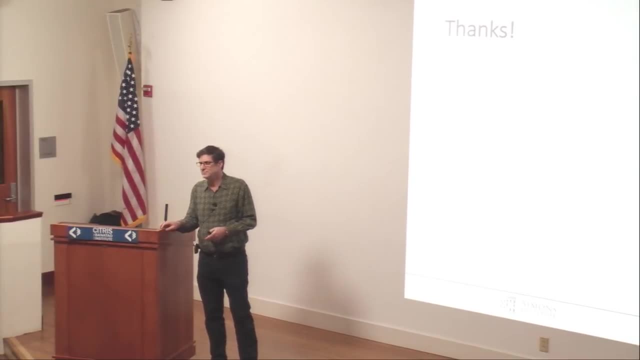 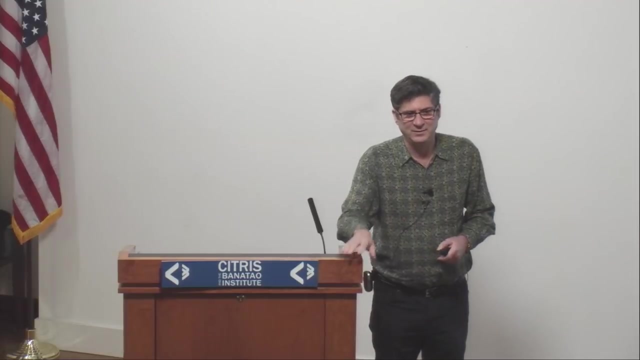 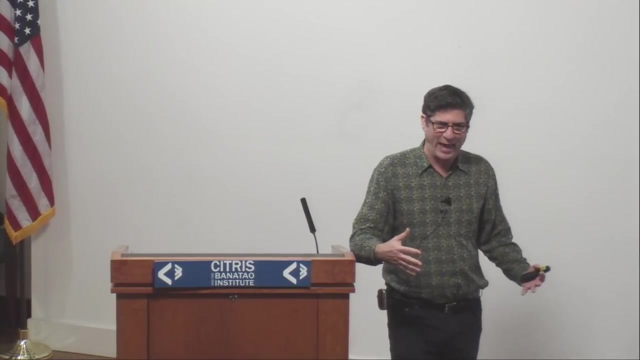 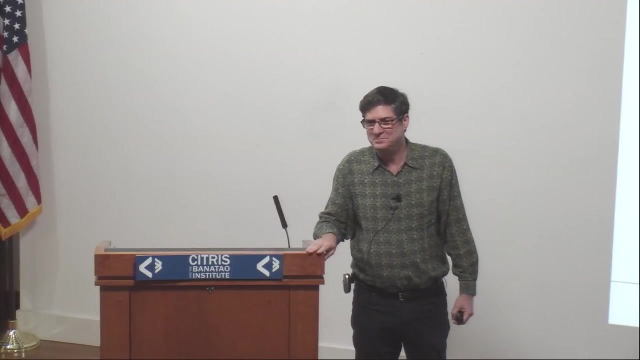 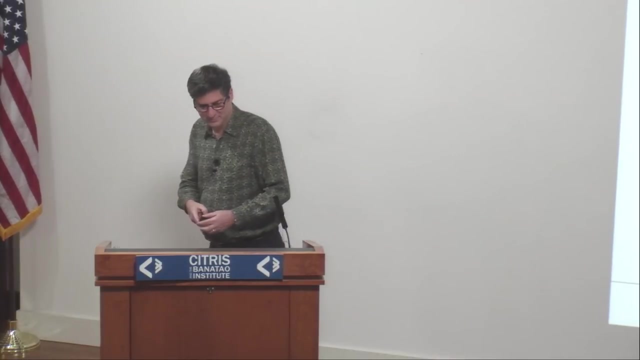 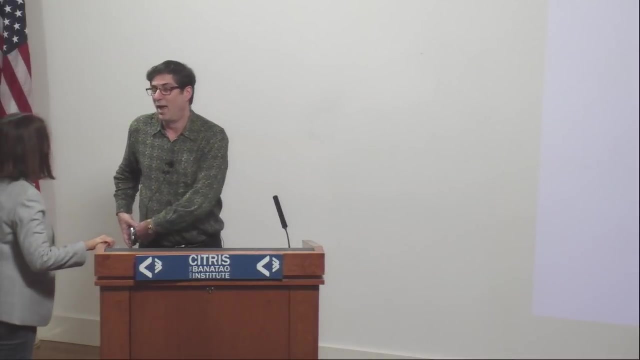 It's pretty interesting, I think So thank you. Well you, the pigeons you saw were pretty fat, I don't know. Thank you, Thank you, So much material. You have material for two hours.